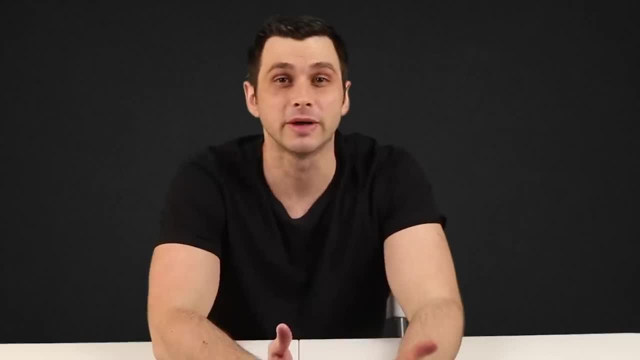 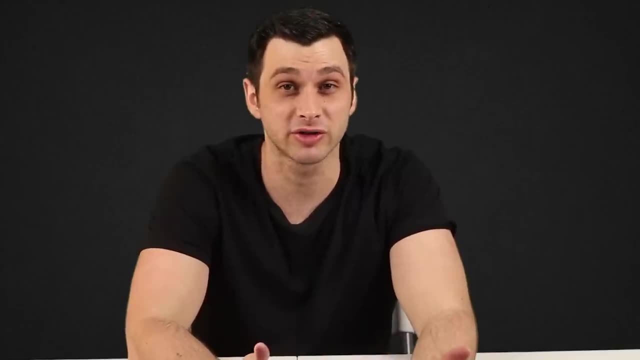 This video is sponsored by Brilliant. Let's just get to the point. Why do we learn differential equations? Because they are the equations that describe how nature works. The universe one day said, boom, here's a bunch of stuff. And we said, cool, how's it all work? 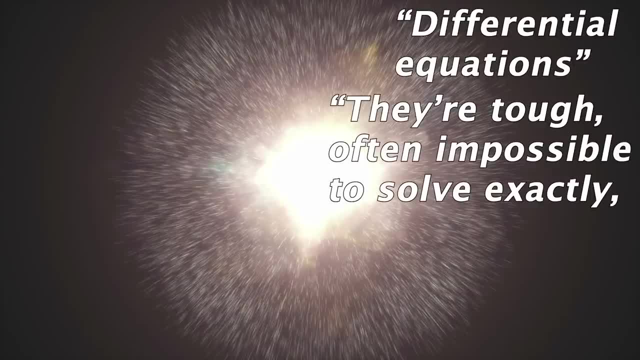 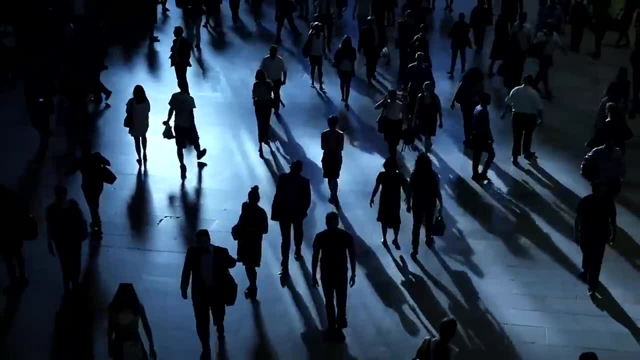 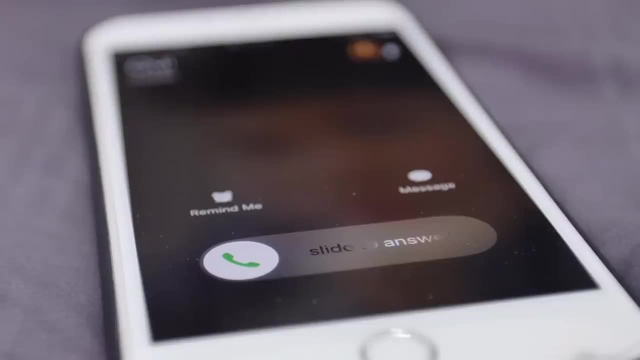 And the universe said: differential equations. They're tough, often impossible to solve exactly, but you'll eventually get some cool stuff from them. Modeling how a population will grow involves differential equations How any fluid moves, differential equations Electromagnetism, which is how phones radio. 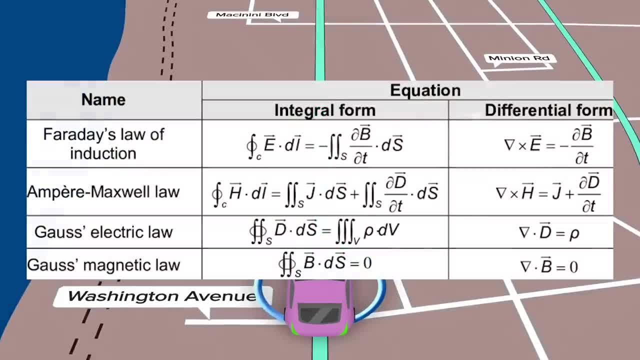 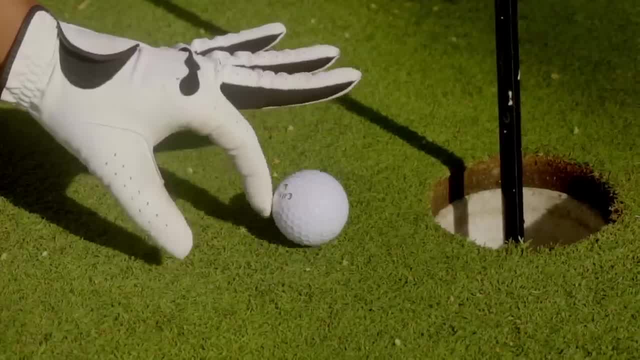 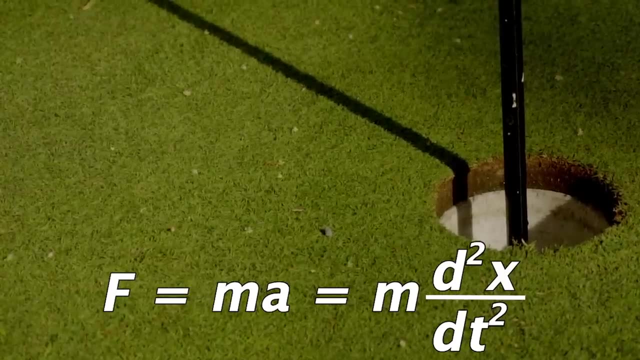 Wi-Fi and GPS all work. Not one, but four differential equations, known as Maxwell's equations. There's electric circuits, and even if something touches something else and thus exerts a force, differential equations are used to describe the motion. If there's no physical contact, like with orbiting bodies, 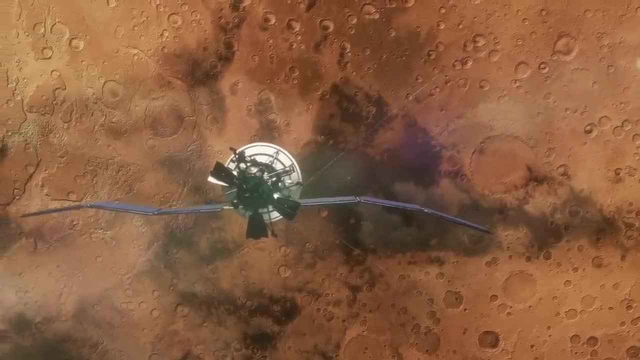 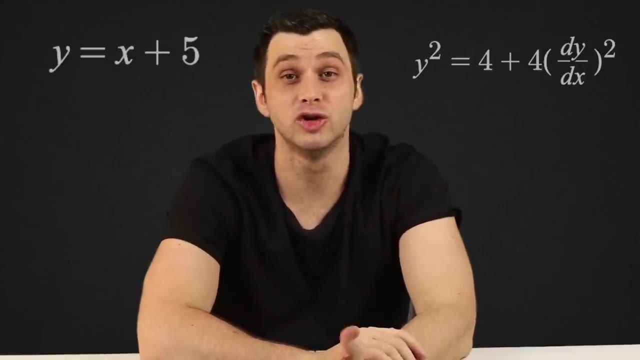 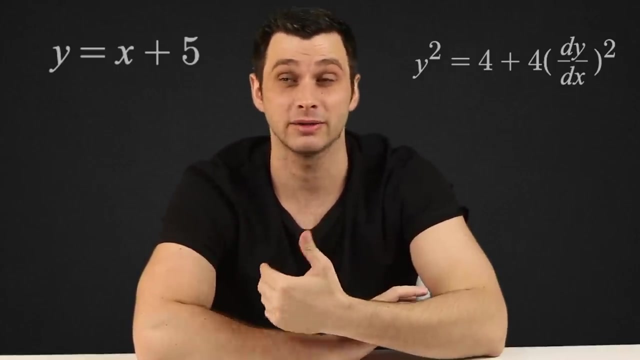 there's still a force, so there's still differential equations. Now, as with simple algebraic equations, differential equations can- and often do, have meaning when you read into the story that they're telling, Like this equation could be saying: my age is Y and I'm exactly five years older. 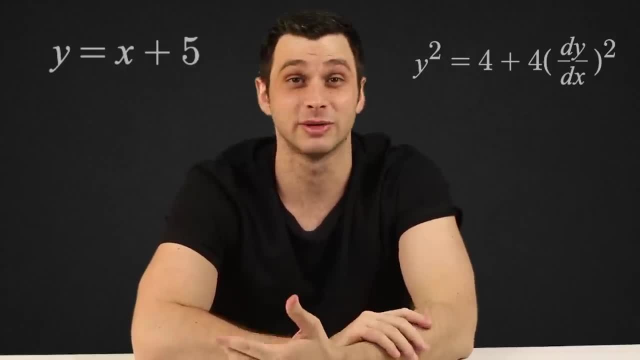 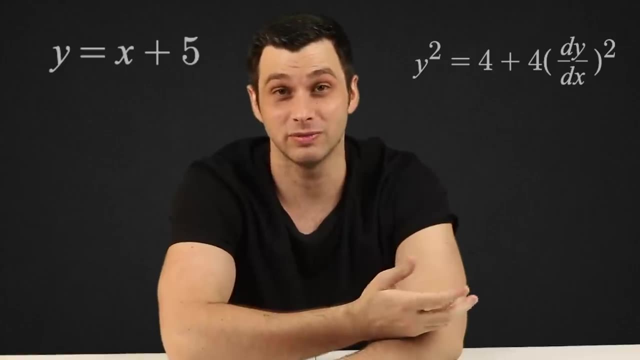 than my brother, whose age is X, And we can use this to determine either of our ages, given the other. Pretty boring, but we can give it meaning. This equation can have meaning too, Or rather, it asks a question, and that question is: 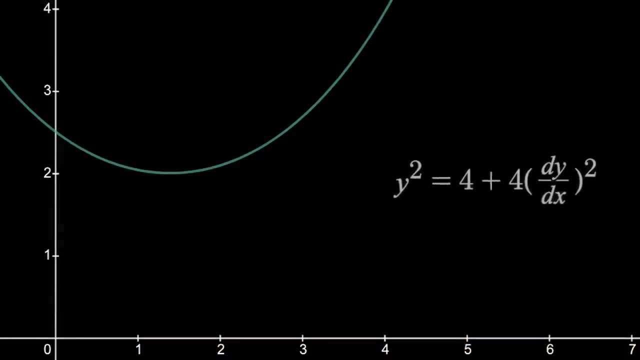 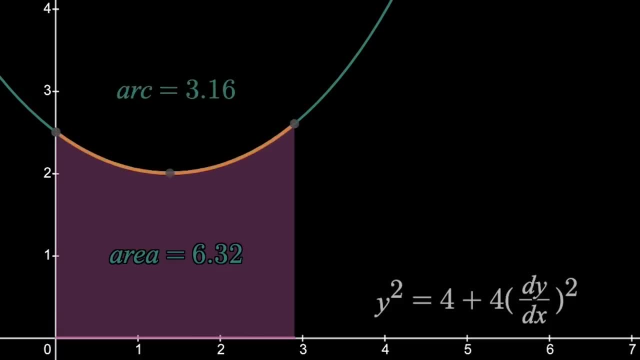 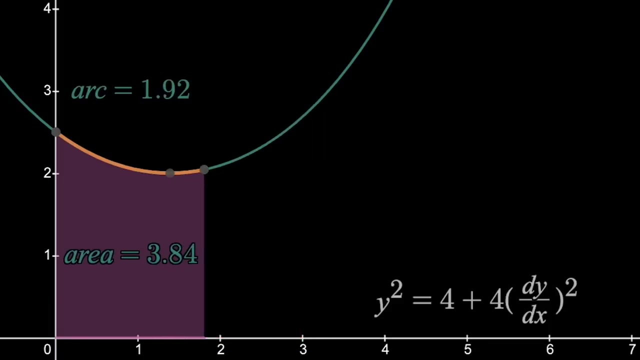 what curve or family of curves have the property where the numerical value of the area under the curve is twice the numerical value of the arc length on that same interval, for any given interval A to B. Well, to set this up, we start with this equation: 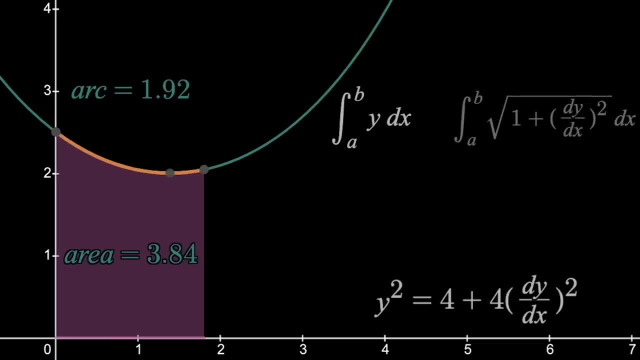 which is the area under the curve itself. And this is the equation for the arc length on that same interval A to B. But we wanna know when the left side always equals twice the right side. Now we can differentiate both sides to remove the integral sign. 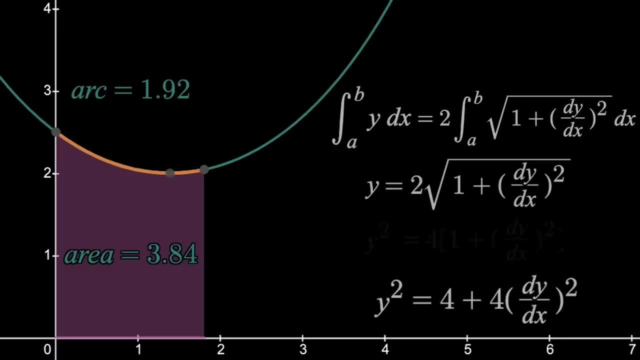 and we're left with a differential equation. From here we can square both sides and then distribute and we get that original equation. If you solve for that function Y, you'd get this, which is the curve you're seeing here. 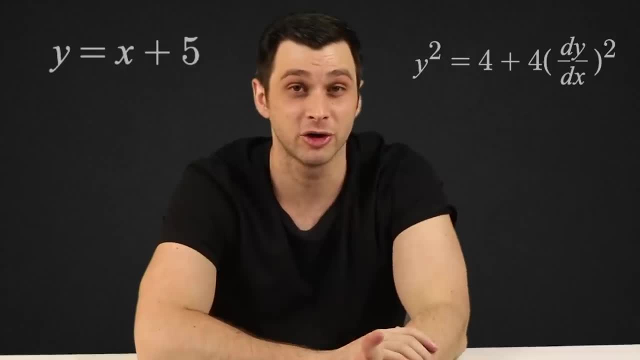 my age is Y and I'm exactly five years older than my brother, whose age is X, And we can use this to determine either of our ages given the other. Pretty boring, but we can give it meaning. This equation can have meaning too. 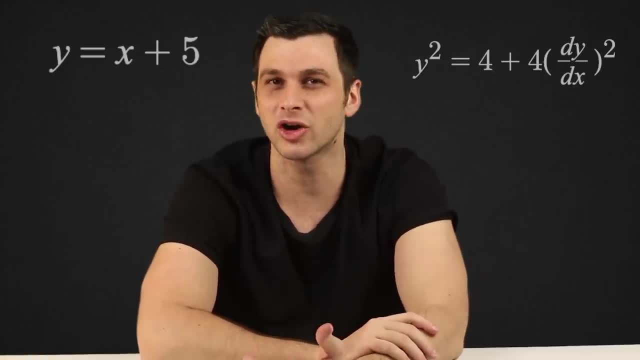 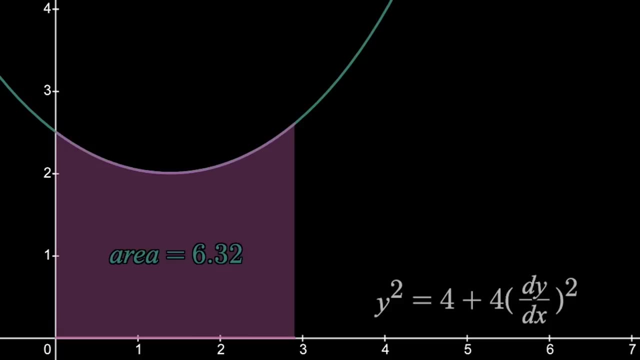 Or rather it asks a question, and that question is: what curve or family of curves have the property where the numerical value of the area under the curve is twice the numerical value of the arc length on that same interval? for any given interval A to B, 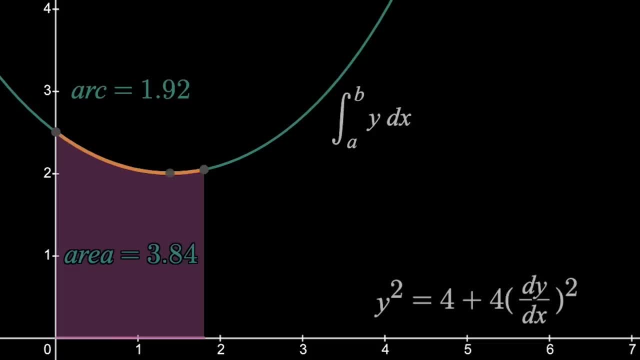 Well, to set this up, we start with this equation, which is the area under the curve itself, And this is the equation for the arc length on that same interval A to B. But we wanna know when the left side always equals twice the right side. 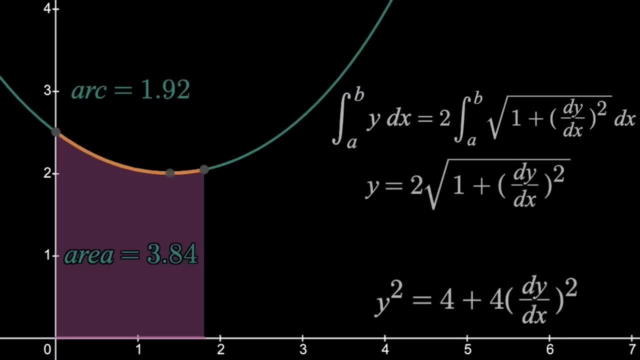 Now we can differentiate both sides to remove the integral sign and we're left with a differential equation. From here we can square both sides and then distribute and we get that original equation. If you solve for that function Y, you'd get this. 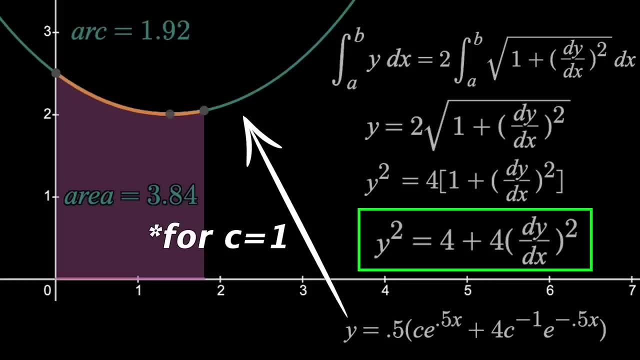 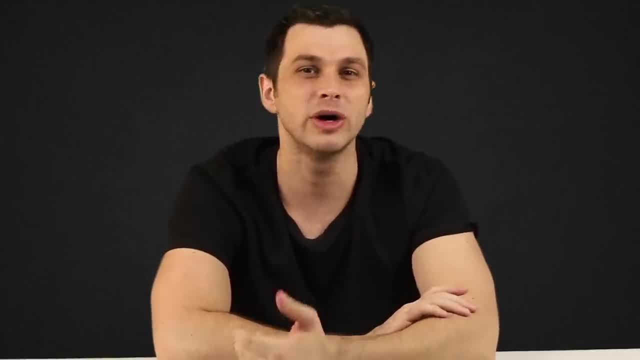 which is the curve you're seeing here. So that's one example of meaning within a differential equation, But let's see how these really describe, so to speak, the value of the arc length. Let's look at some real-world situations, because it's not always obvious. 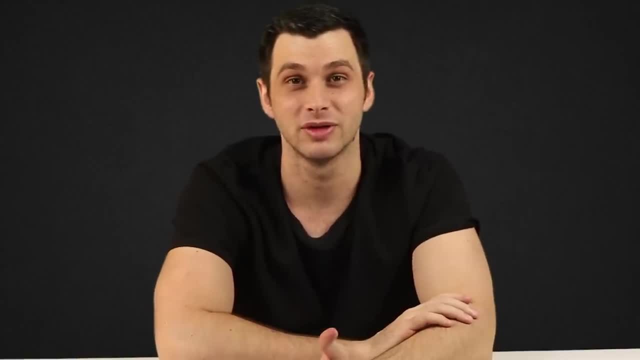 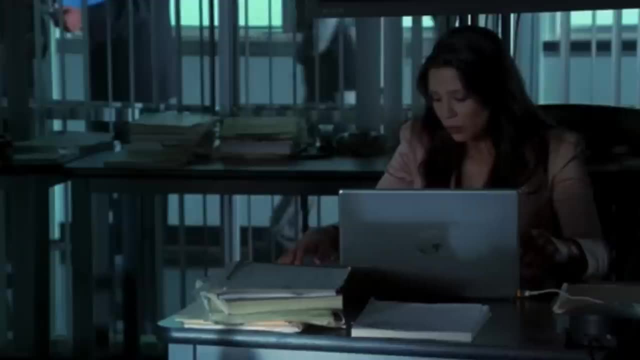 what story these equations tell or how they show up in general. And since I always love bringing up the TV show Numbers when I can, here's a perfect example. So check out this scene from an episode where law enforcement is trying to catch a couple. 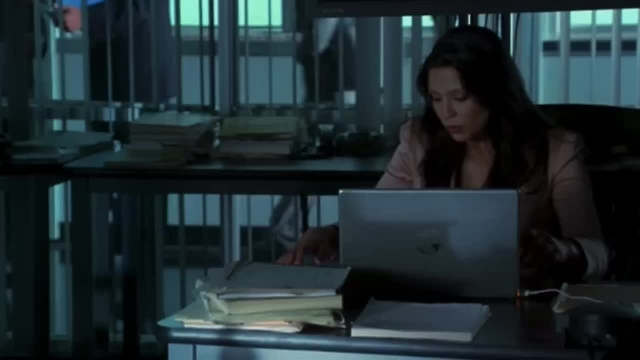 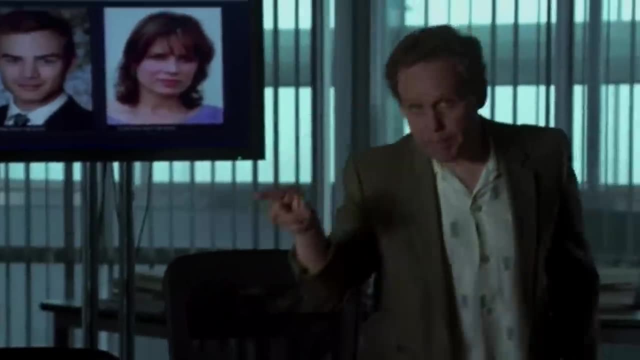 committing crimes as they travel across the United States. When we plot your movements against those that are targets, the pattern makes itself known. And when we plot your path against oil in winter, we're gonna have a pattern that makes itself known. And when we plot your path against oil in winter, 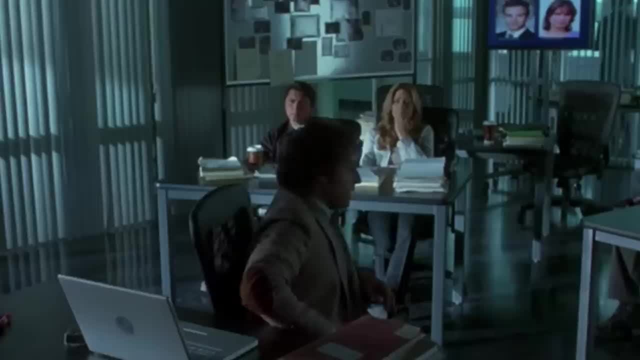 we're gonna have a pattern that makes itself known. And when we plot your path against oil in winter, we got this. Yeah, this is the Red Desert robbery, The missing point on a curve that I didn't even realize I was looking at. 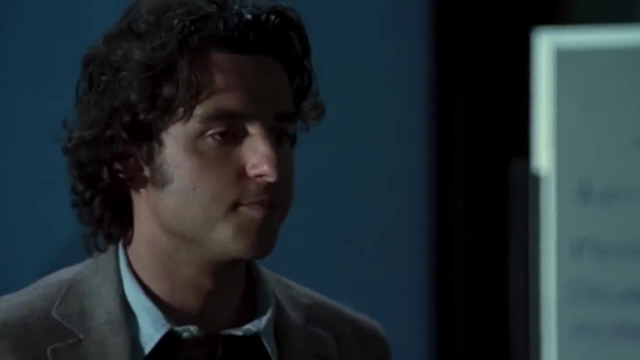 It's a variation on something called a pursuit curve. All right, so what's happening here is the FBI has been chasing this couple across the country, but hasn't caught them yet, So the mathematicians plotted the path both the criminals and the FBI took. 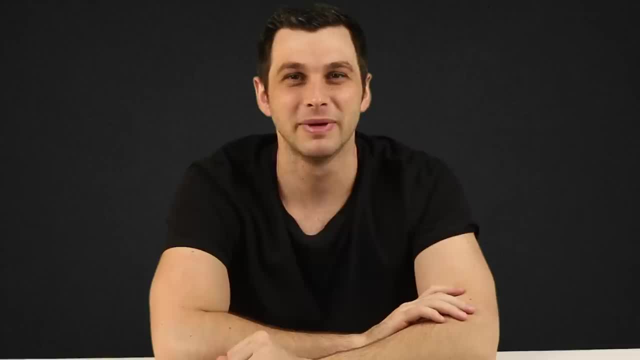 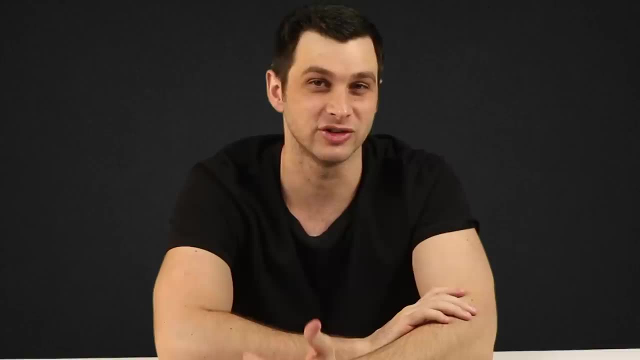 So that's one example of meaning within a differential equation. But let's see how these really describe the difference. but let's see how these really describe the difference, some real world situations, because it's not always obvious what story these equations tell or how they show up in general, And since I always love bringing up the tv show numbers when I can, 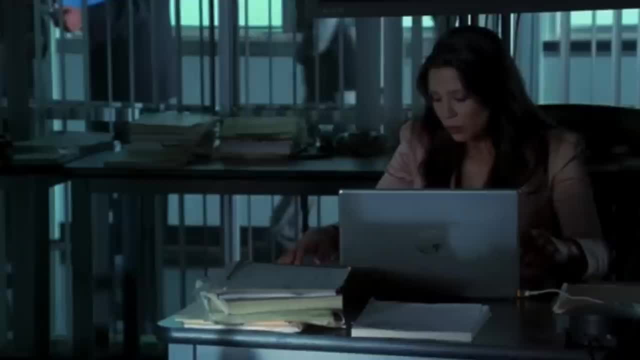 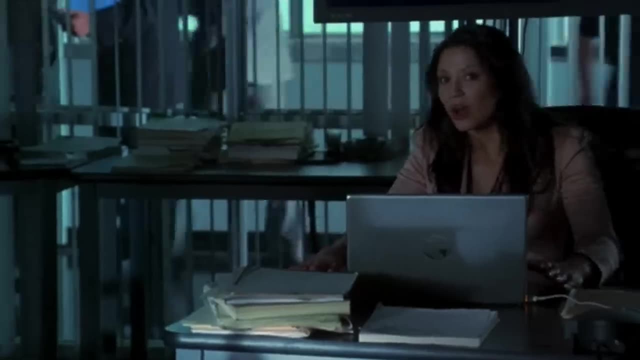 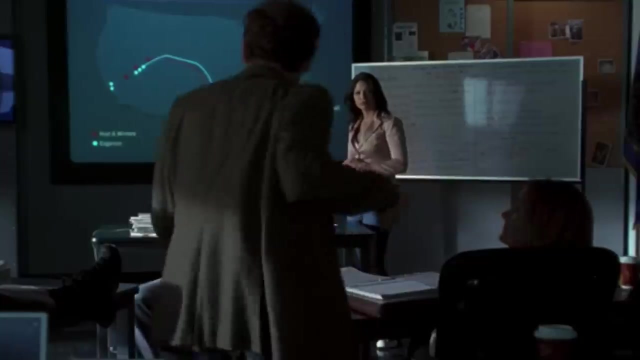 here's a perfect example. So check out this scene from an episode where law enforcement is trying to catch a couple committing crimes as they travel across the United States. When we plot your movements against those of your targets, the pattern makes itself known. And when we plot your path against oil and winters, we got this. 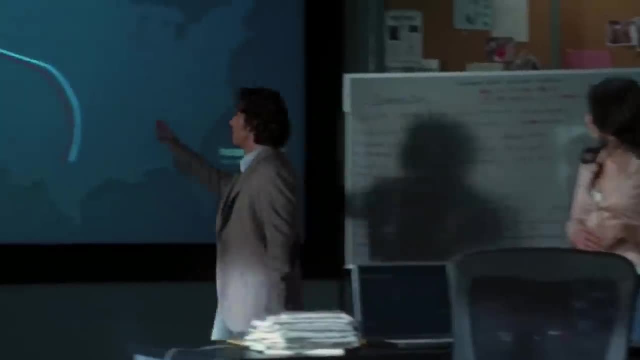 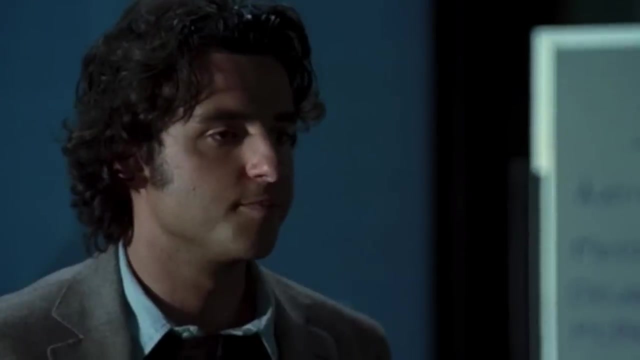 Yeah, this is the red desert robbery. The missing point on a curve that I didn't even realize I was looking at. It's a variation on something called a pursuit curve. All right, so what's happening here is the FBI has been chasing this couple across the country, but hasn't caught them yet, So the 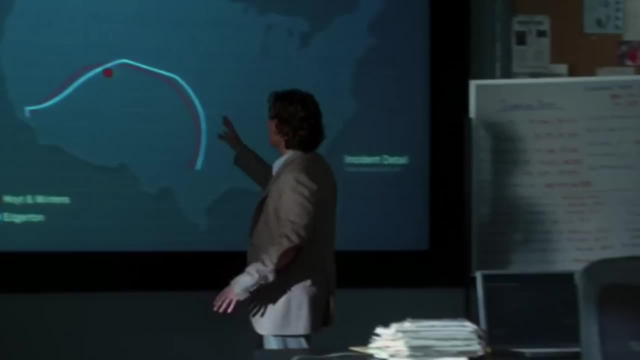 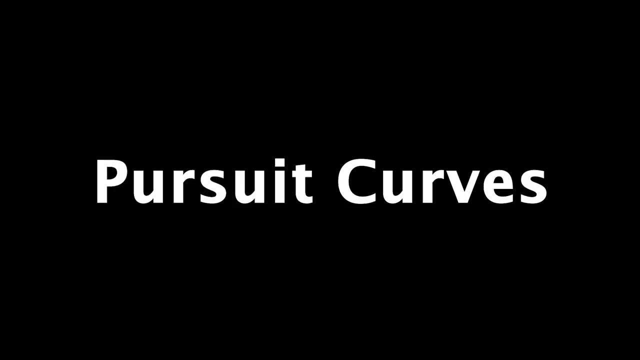 mathematicians plotted the path both the criminals and the FBI took to the to see if they can make some predictions about where the criminals will strike next, And this is related to pursuit curves. A pursuit curve is simply the curve traced out by one object chasing another, although there are usually conditions listed for something to be technically 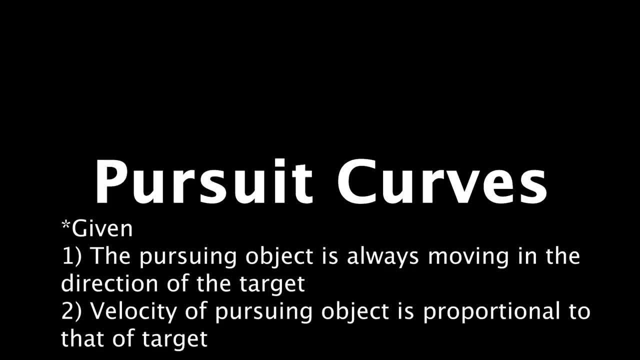 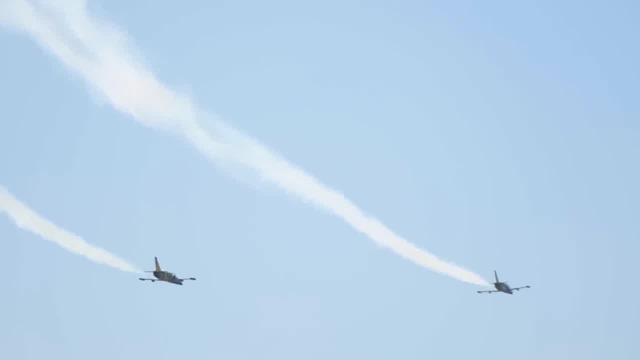 considered a pursuit curve. But this could apply to a cheetah chasing down a gazelle, or one aircraft chasing another, for example. So let's see how we can determine the curve that the pursuing object will be chasing. So let's see how we can determine the curve that the pursuing object 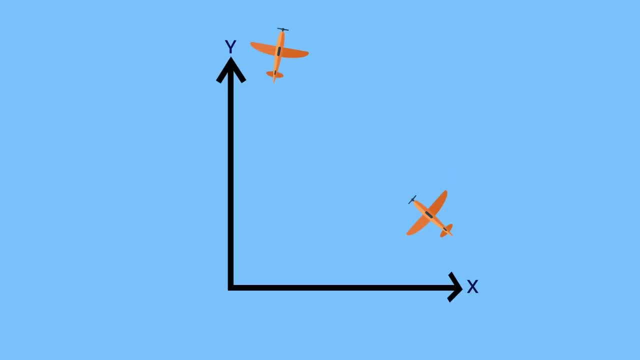 will be chasing. So let's see how we can determine the curve that the pursuing object will trace out. Now two things to note. First, we're going to assume that the plane being chased has a predetermined path, whether it's flying straight up or in a circle or whatever. 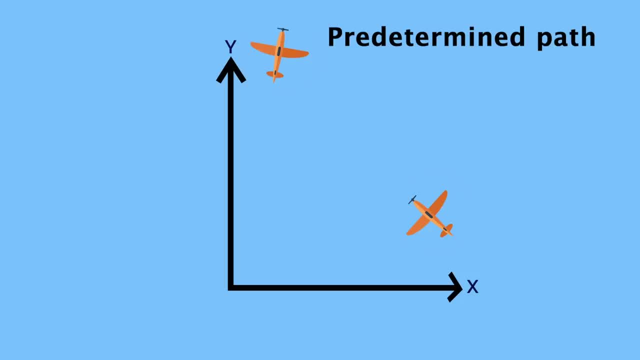 Assume we already know their path. Then the second assumption, like I mentioned before, is that the chasing object is always moving in the direction of the other and it turns its nose as needed during pursuit. In reality, this could be like a plain one eye他x обычных躲 UV手���male zu einer Shoulder. In reality this could be like a plain one eyeťah at one 26 00m uhr: amlifarten und sich čar ładen. In reality this could be like a plain one eyeťah at one 26 00m uhr: amliferen unter BBQreeų nr. 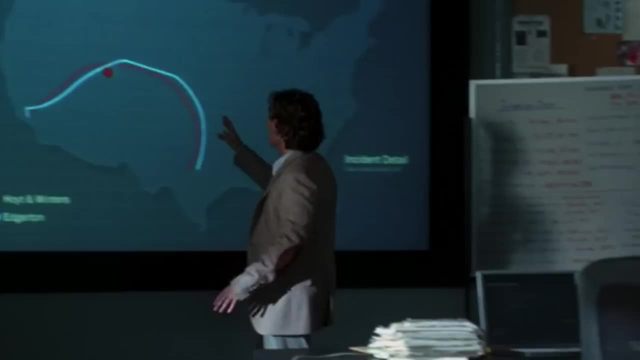 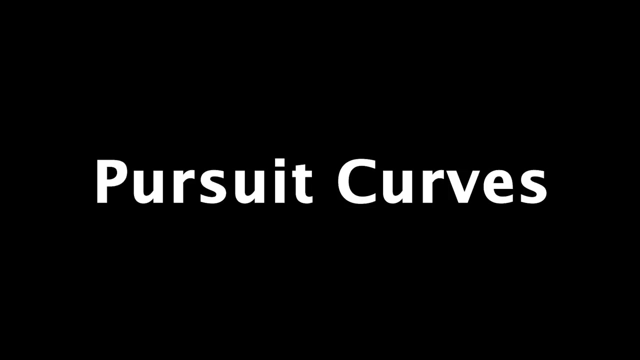 to see if they can make some predictions about where the criminals will strike next, And this is related to pursuit curves. A pursuit curve is simply the curve traced out by one object chasing another, although there are usually conditions listed for something to be technically considered a pursuit curve. 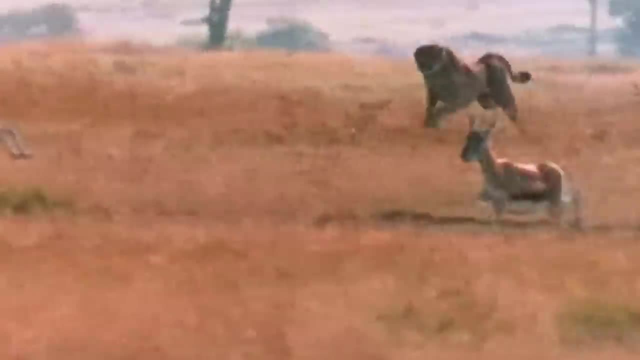 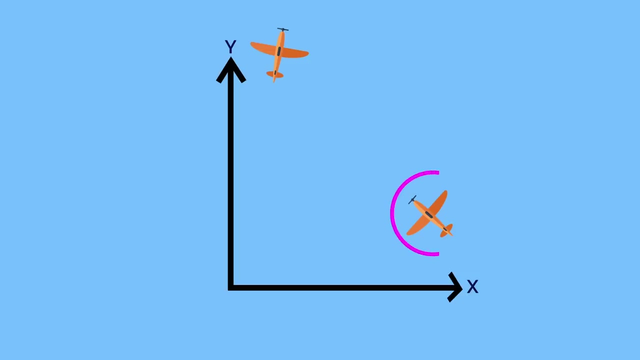 But this could apply to a cheetah chasing down a gazelle, or one aircraft chasing another, for example. So let's see how we can determine the curve that the pursuing object will trace out. Now, two things to note. First, we're going to assume that the plane being chased 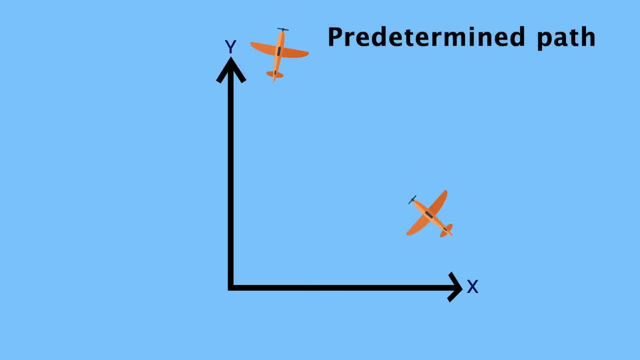 has a predetermined path, Whether it's flying straight up or in a circle or whatever- assume we already know their path. Then the second assumption, like I mentioned before, is that the chasing object is always moving in the direction of the other and it turns its nose as needed during pursuit. 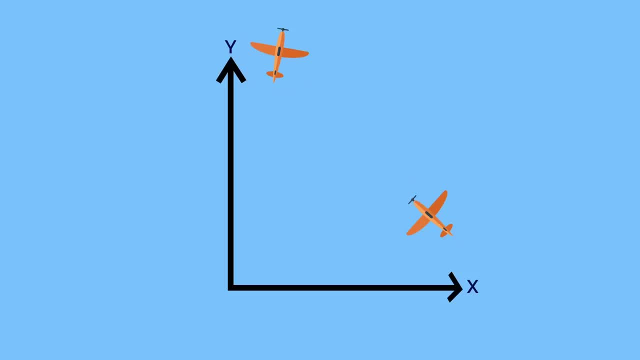 In reality, this could be like a plane wanting its forward-facing guns on the ground, but it's always aimed at the target, or something. Anyways, what you're seeing here is a snapshot of the chase, and we can represent the current positions of each plane. 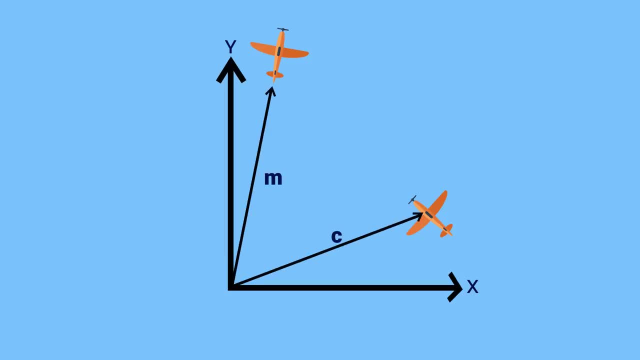 with a vector, I'll say C and M for cat and mouse. The other thing we know is that at this time, or really any time, the chasing plane is pointed at the front one which means this is their velocity vector, or C prime at this moment. 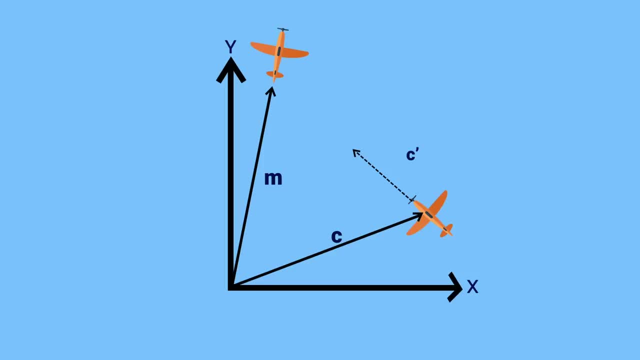 There's no wind or anything, so the plane is definitely flying in the direction it's pointed. Now we don't know the speed or the length of that vector currently, but we know the direction at least. That's more important, because there's another vector. 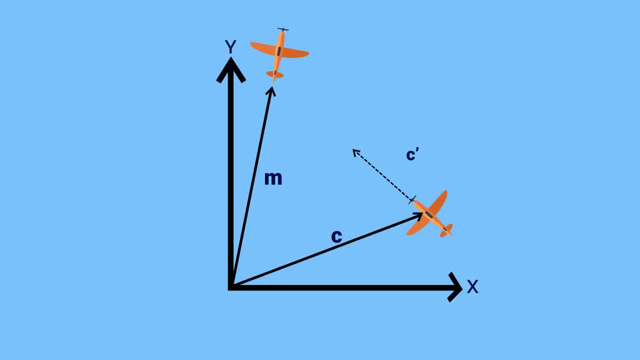 pointing in that same direction, which is easy to find, and that's M minus C. For the visualization, M minus C is the same as M plus negative C, and putting negative C on top of M gives us a vector that points from the back plane to the front one. 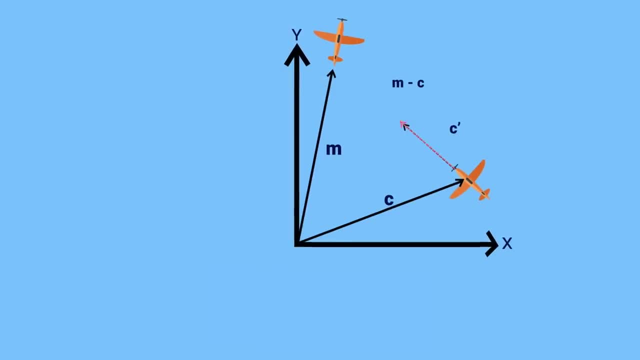 Then to deal with the lengths, I'm going to normalize the two vectors by dividing by their magnitudes, so they both have a length of one. This is key because the dot product of two vectors, both with length one and pointing in the same direction. 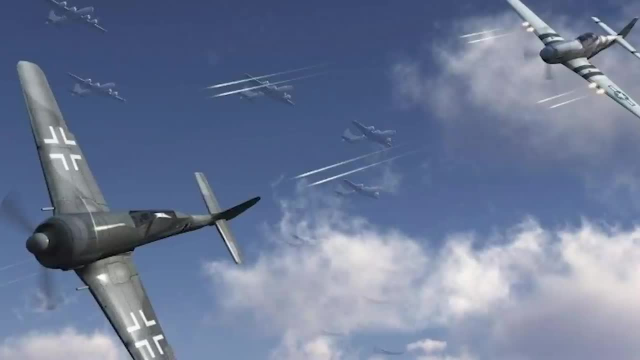 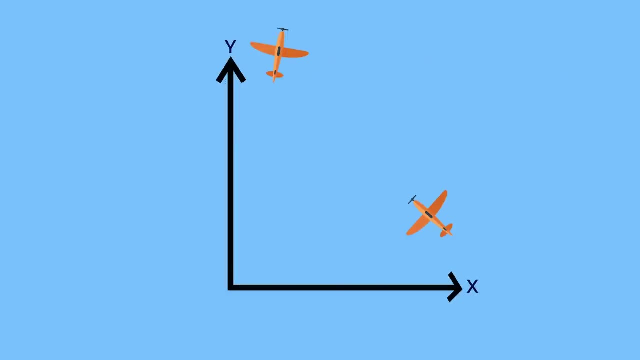 be like a plane wanting its forward-facing guns always aimed at the target, or something. anyways, what you're seeing here is a snapshot of the chase, and we can represent the current positions of each plane with a vector. i'll say c and m for cat and mouse. 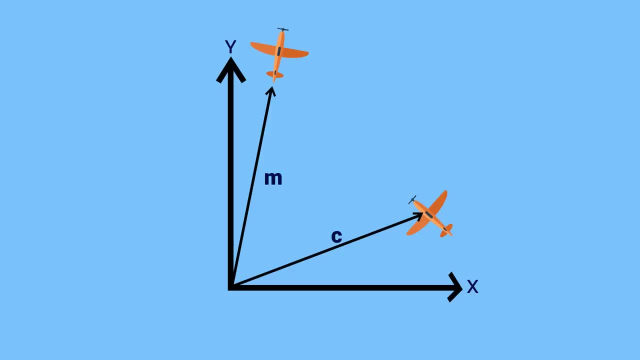 the other thing we know is that at this time, or really any time, the chasing plane is pointed at the front one, which means this is their velocity vector, or c prime. at this moment there's no wind or anything, so the plane is definitely flying in the direction it's pointed. now we don't know the speed or the length of that vector. currently, 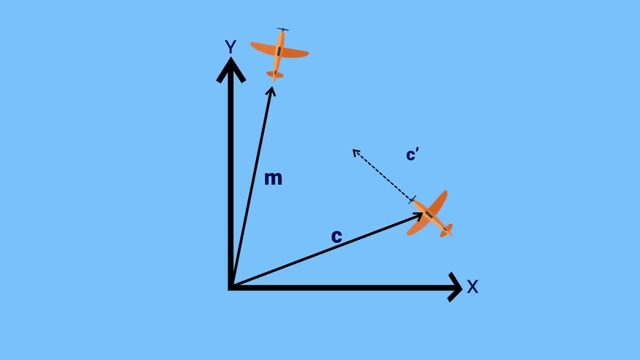 but we know the direction at least. that's more important because there's another vector pointing in that same direction, which is easy to find, and that's m minus c. for the visualization, m minus c is the same as m plus negative c, and putting negative c on top of m, 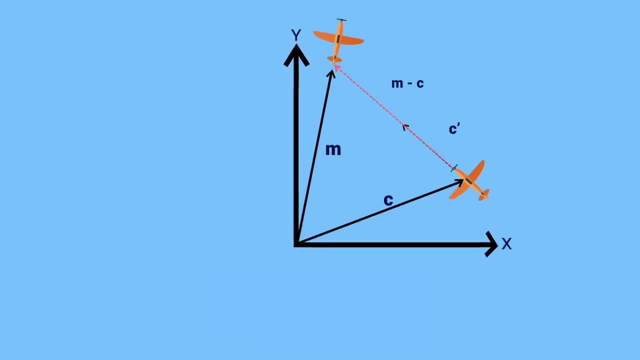 gives us a vector that points from the back plane to the front one. then to deal with the lengths, i'm going to normalize the two vectors by dividing by their magnitudes, so they both have a length of one. this is key because the dot product of two vectors 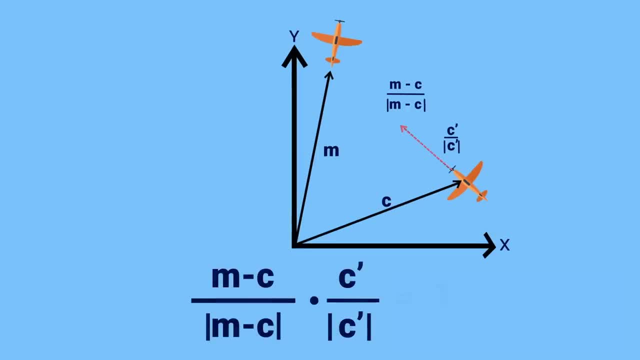 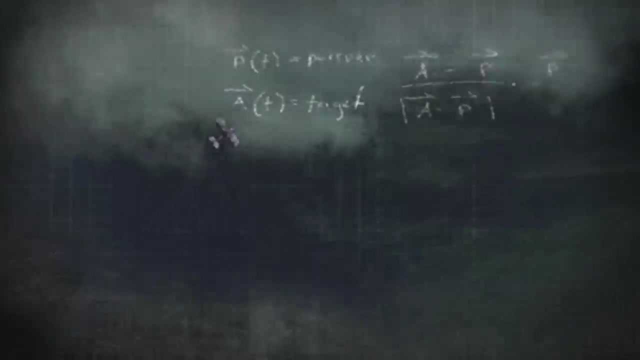 both with length one and pointing in the same direction is one. this is a fundamental equation. yes, i could have just set the vectors equal to one another, but i'm doing this because in that episode i'm going to be talking about how to solve the m-vector, so that you can see that equation. 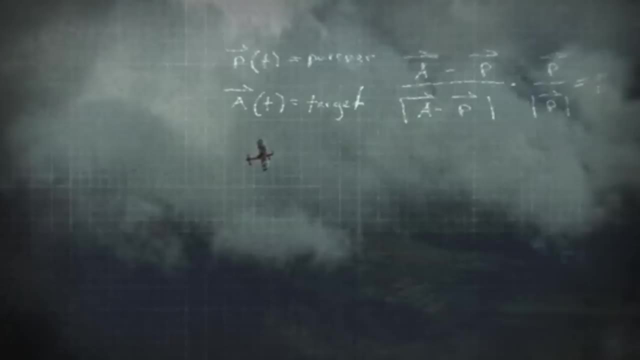 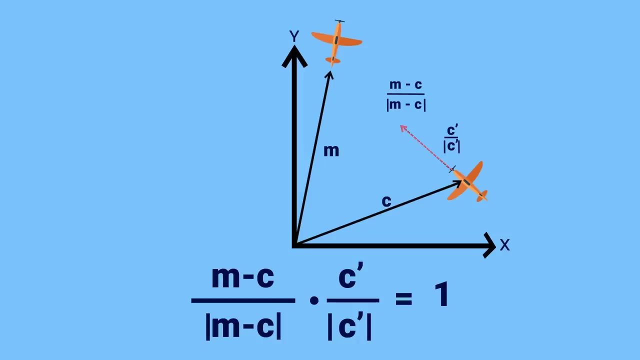 when you're reading mathematics or you're a mathematician, is explaining pursuit curves. you can see that equation come on the screen. so now you know the meaning behind it, but still it's not really obvious how to solve it yet. but if we go back to our snapshot, remember 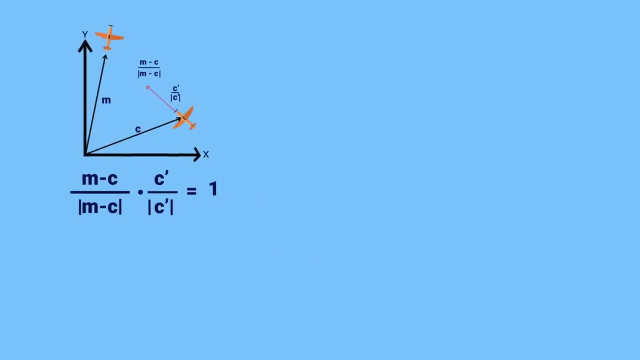 that the m vector is actually a known function of time. we're seeing it only at one moment in time, but it is changing as the planes fly around. so i'll say it's a vector function. u of t, comma, v of t. The c vector also changes in time, but it's our unknown. 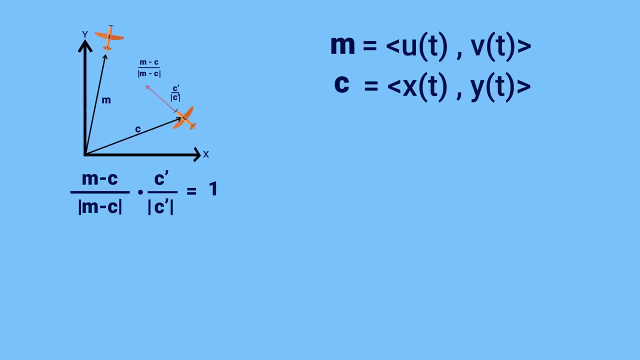 some x of t, comma y of t that we want to solve for, And the c prime vector would just be x prime of t, comma y prime of t. So then m minus c would give us this vector, here just the x component subtracted. 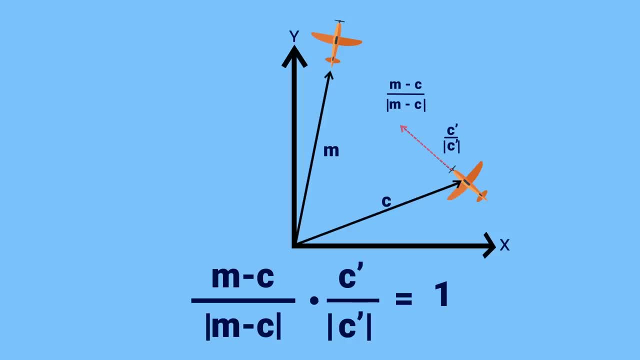 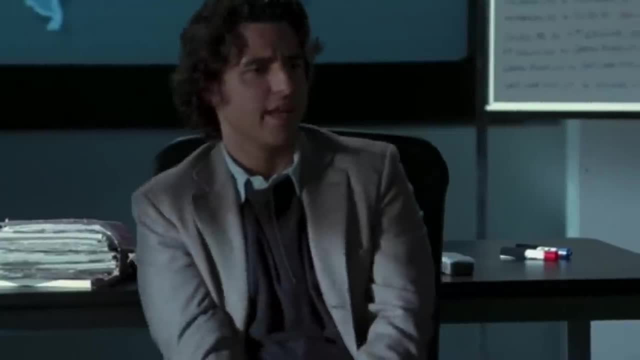 is one. This is a fundamental equation. Yes, I could have just set the vectors equal to one another, but I'm doing this because in that episode, when the mathematician is explaining pursuit curves, you can see that equation come on the screen. 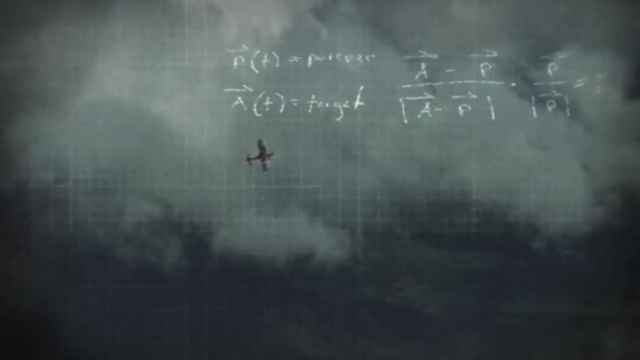 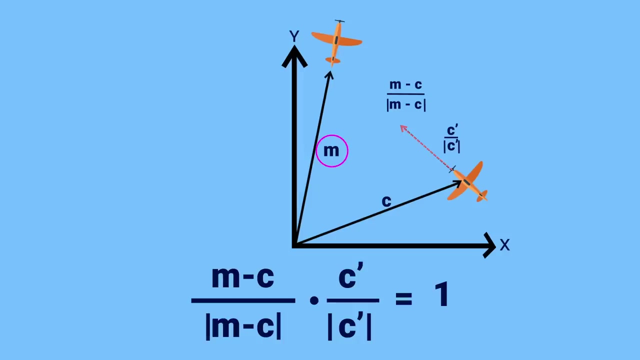 so now you know the meaning behind it, But still it's not really obvious how to solve it yet. But if we go back to our snapshot, remember that the M vector is actually a known function of time. We're seeing it only at one moment in time. 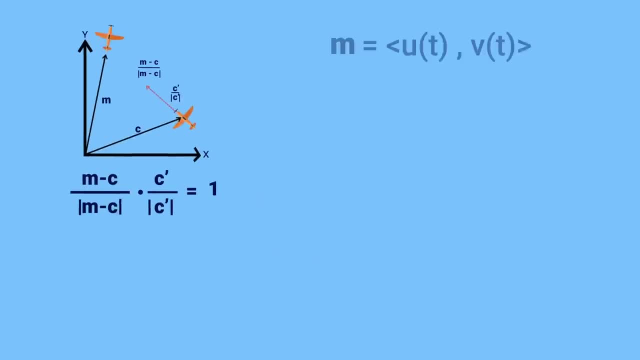 but it is changing as the planes fly around. So I'll say it's a vector function u of t, comma v of t, which are both known. I'm just keeping things generic. The C vector also changes in time, but it's our unknown. 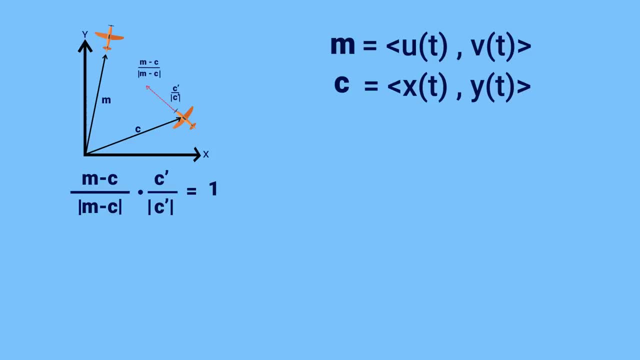 It's the x of t comma y of t that we want to solve for, And the C prime vector would just be x prime of t, comma y prime of t. So then M minus C would give us this vector, here Just the x component subtracted. 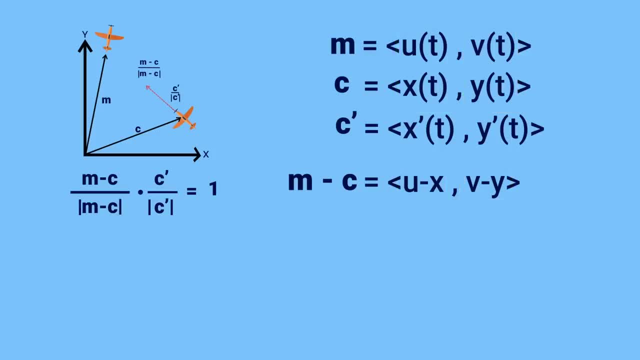 and the y component subtracted, And I'm just not writing the t's, so there's room. I'll do the same thing with C prime. Then if we plug all of those into our equation that we want to solve, we get this. 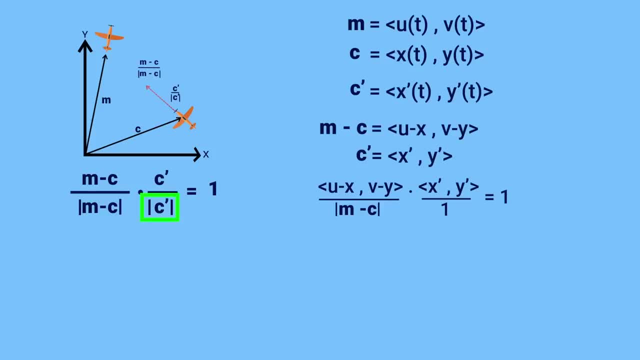 Now, the one extra thing I did is assume the magnitude of C prime to one, Which just means we assume the chasing plane is flying at a constant speed of one. just to simplify the equation, Then we just have to do the dot product, which leaves us with this differential equation. 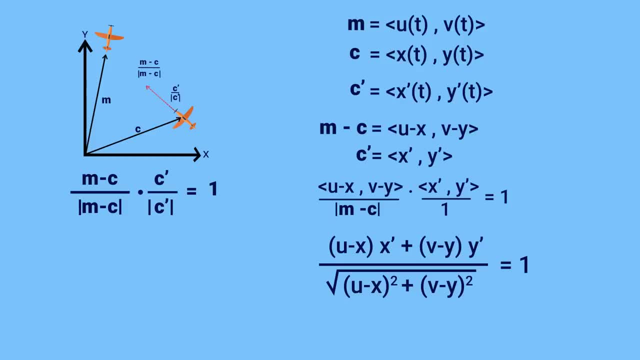 You'll notice, I actually wrote out the expression for the magnitude of M minus C on the bottom here. The only problem with this is that there are two unknown functions, x and y, in this equation, But that would just be the one saying the chasing plane is flying. 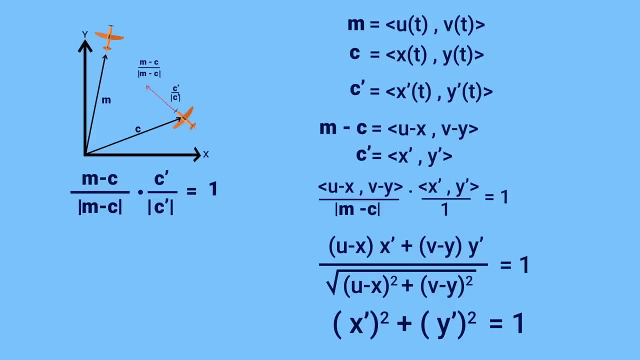 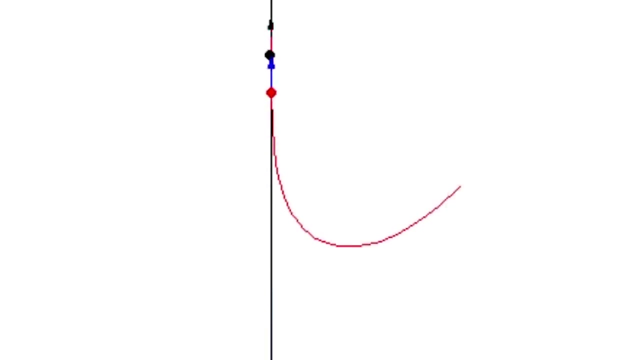 at a constant speed of one. Now we have a system of differential equations that can be solved. If, for example, we assume the target plane is flying straight along the y-axis, then this would be the path of the chasing plane shown in red If the target plane were flying in a circle. 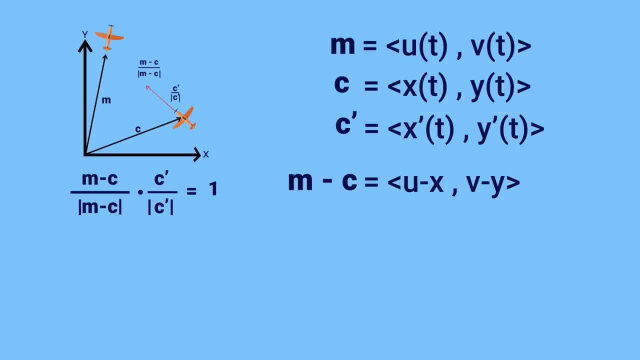 and the y component subtracted And I'm just not writing the t's. so there's room. I'll do the same thing with c prime. Then if we plug all of those into our equation we want to solve, we get this Now. the one extra thing I did was set. 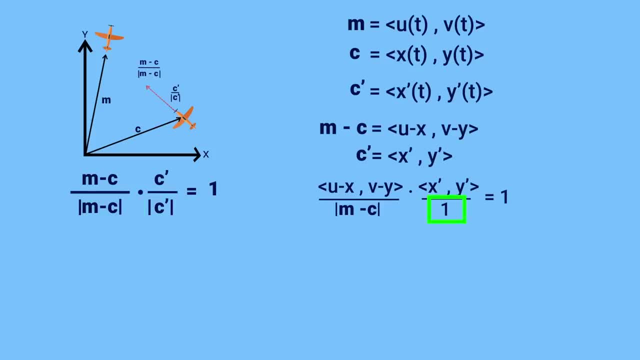 the magnitude of c prime to one, which just means we assume the chasing plane is flying at a constant speed of one. just to simplify the equation, Then we just have to do the dot product, which leaves us with this differential equation. You'll notice, I actually wrote out the expression. 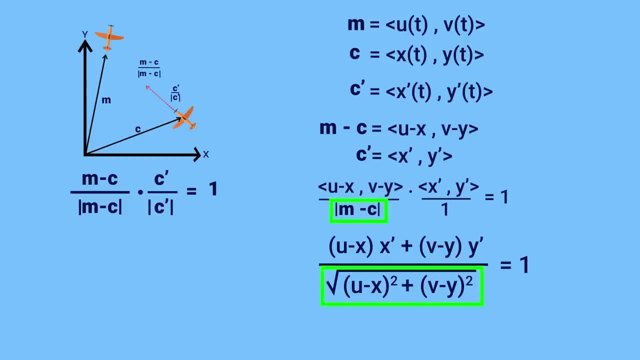 for the magnitude of m minus c on the bottom here. The only problem with this is that there are two unknown functions, x and y, which means we need another equation, But that would just be the one saying the chasing plane is flying at a constant speed of one. 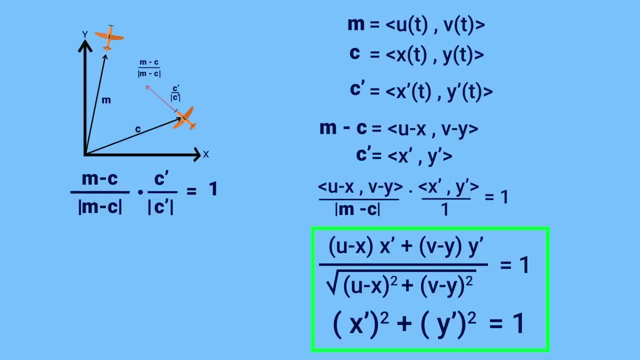 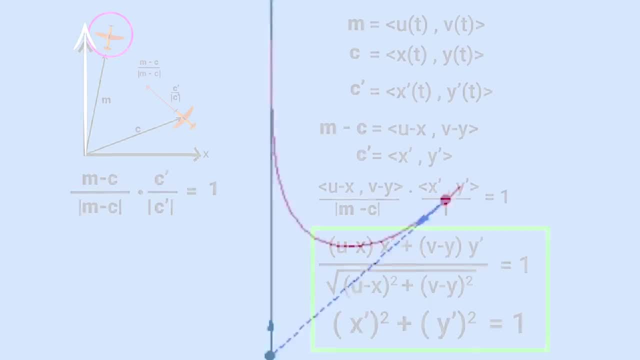 Now we have a system of differential equations that can be solved. If, for example, we assume the target plane is flying straight along the y-axis, then this would be the path of the chasing plane shown in red If the target plane were flying in a circle. 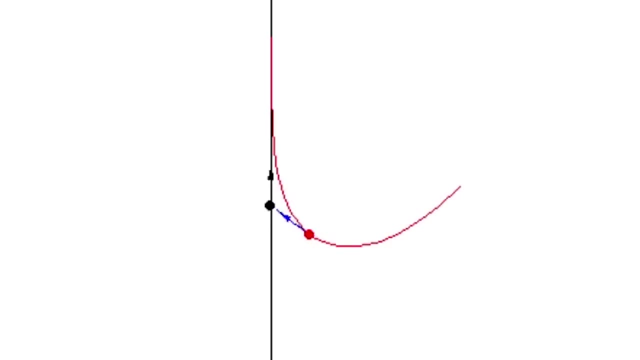 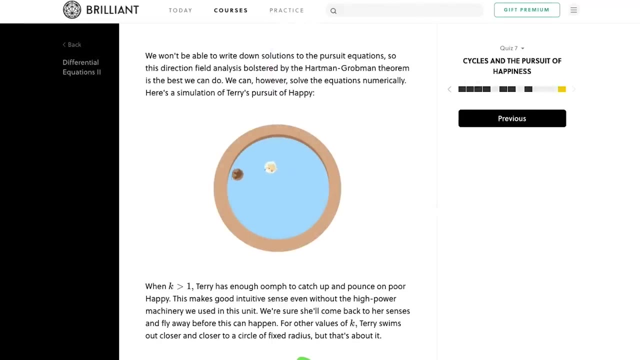 then you'd get something very different shown here on BrilliantSight. Now you'll notice this method of chasing someone isn't necessarily ideal for catching them, but there seems to be other types or variations of pursuit curves that range from always aiming at the target. 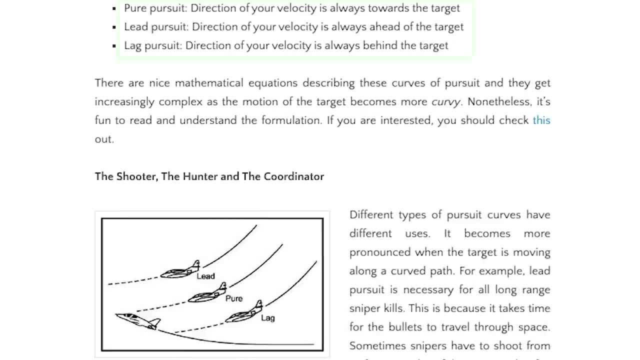 to predicting where they'll go next. On that numbers episode, the situation was more complex, as we saw in the previous video. The target plane was flying at a constant speed of one and the target plane was flying at a constant speed of one. 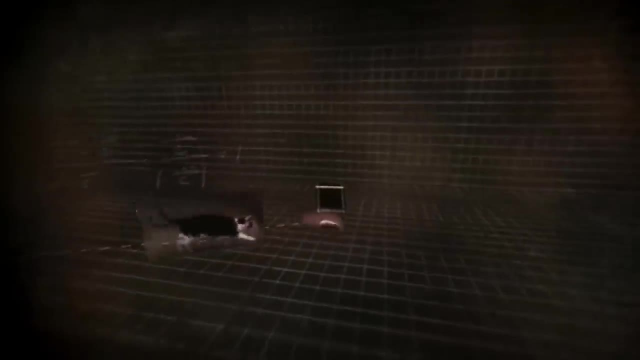 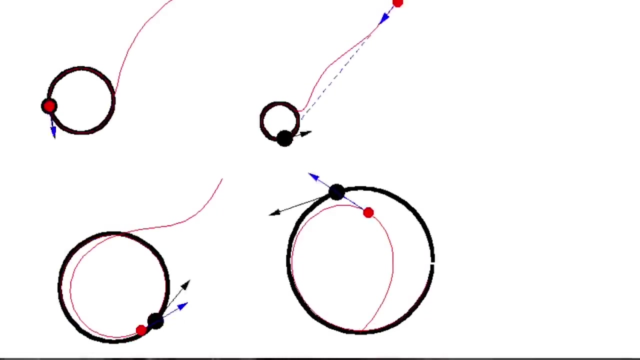 As the mathematicians were accounting for how the moves of the FBI might affect the criminals that were being chased. But still the basics of pursuit curves can be seen in a first level differential equations course And while this might not be a real world, FBI case pursuit curves. 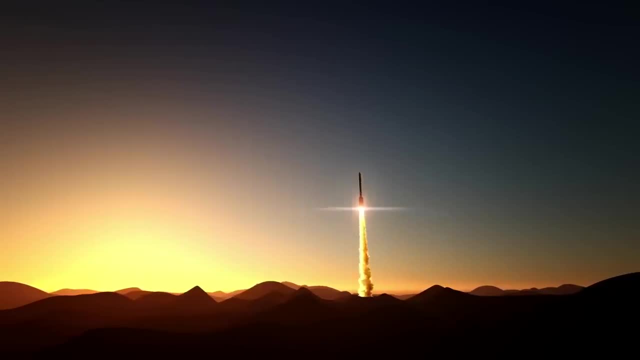 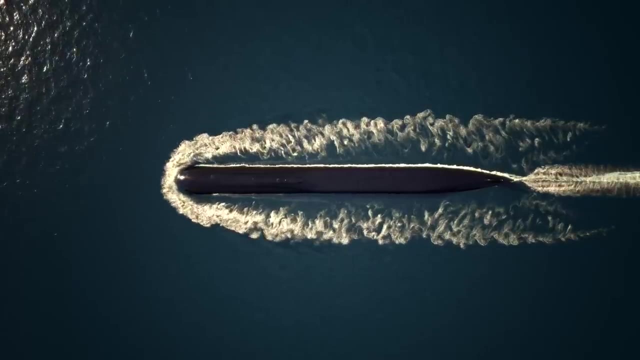 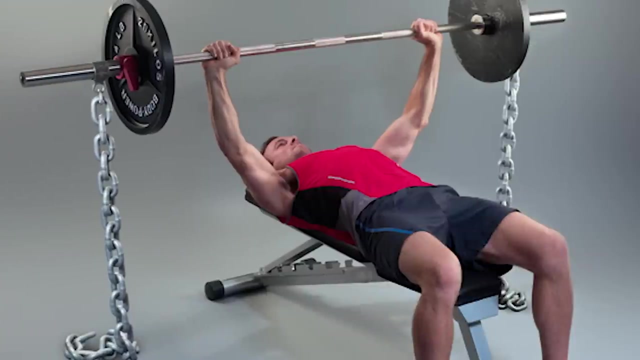 can be applied to missile guidance systems, aircrafts, submarines and so on. Alright, now let's look at something more casual. If you go to the gym, you may have seen or done a bench press or squat with chains hanging off the sides. 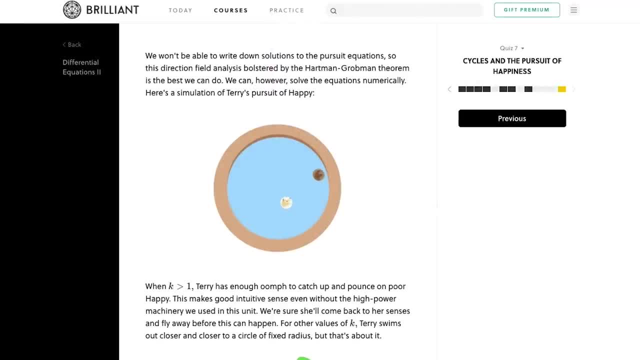 then you'd get something very different, something like this on BrilliantSight. Now you'll notice this method of chasing someone isn't necessarily ideal for catching them, but there seems to be other types or variations of pursuit curves that range from always aiming at the target. 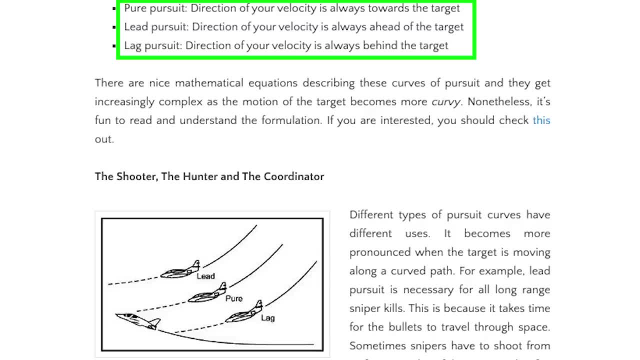 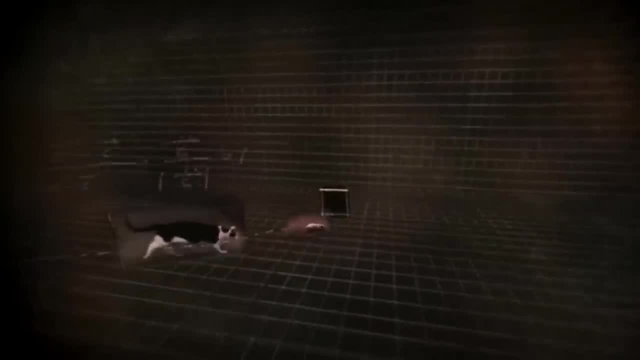 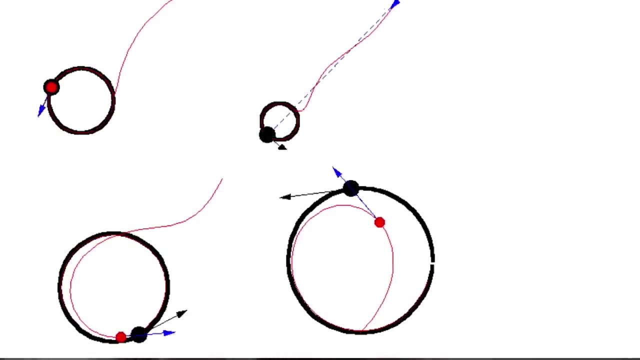 to predicting where they'll go next. On that numbers episode, the situation was more complex as the mathematicians were accounting for how the moves of the FBI might affect the criminals that were being chased. But still the basics of pursuit curves can be seen in a first level differential equations course. 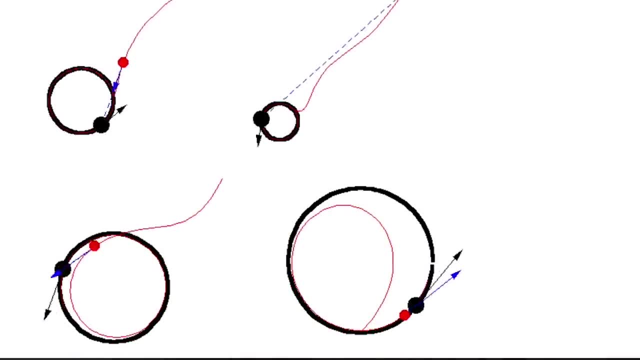 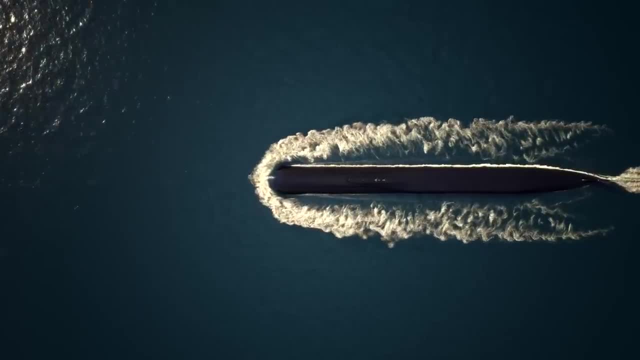 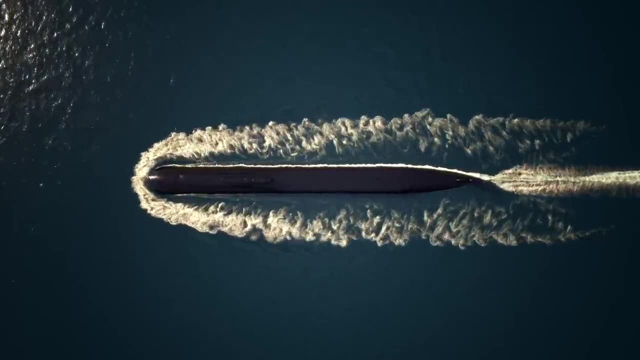 And while this might not be a real world FBI case, pursuit curves can be applied to missile guidance systems, aircraft, submarines and so on. Alright, now let's look at something more casual. If you go to the gym, you may have seen or done. 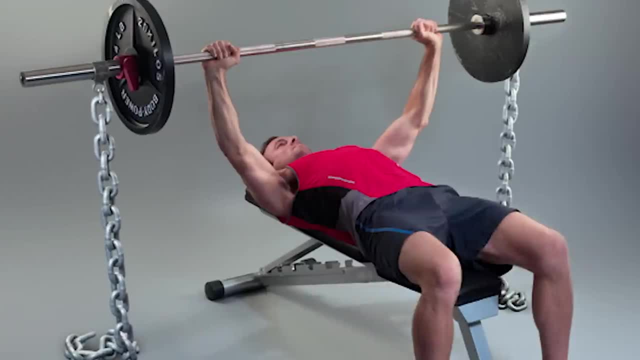 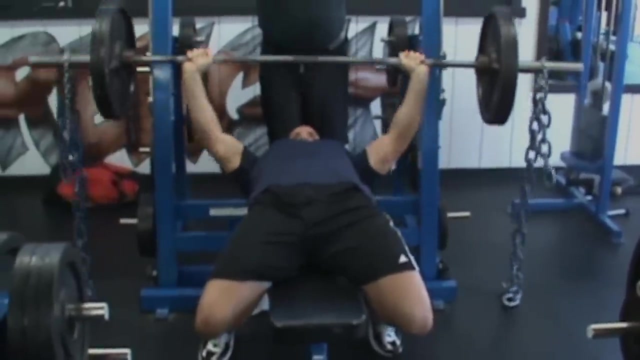 a bench press or squat with chains hanging off the sides. This makes it so that, as the bar moves up, the chain is more and more suspended and thus contributes more of its weight to the exercise, Meaning: as the person pushes upwards, the weight increases. This actually complicates. 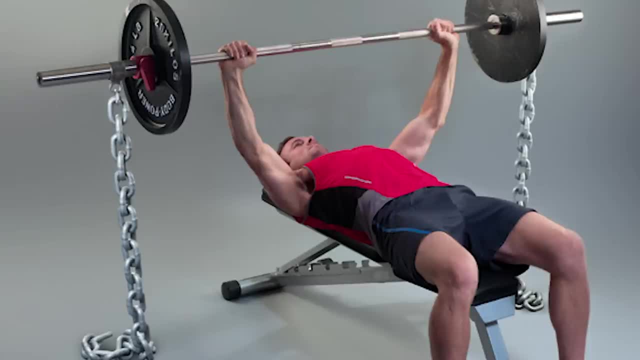 the equation of motion more than you might think, Because for every little dx or change in height, there's a dm or small change in mass in regards to the part of the chain that's off the ground. So let's see what this setup would look like. 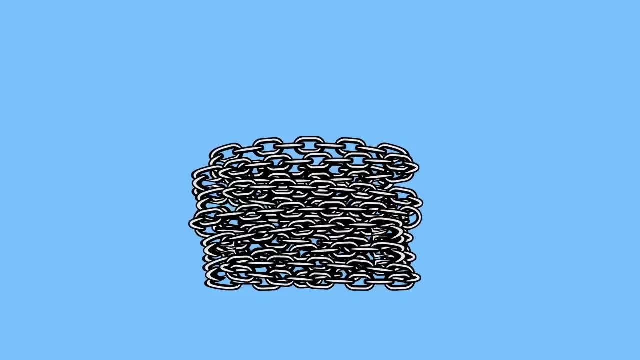 Now we'll say the barbell has no mass, just to make things easier. So really we're just lifting the chain off the ground And we'll call that distance off the ground x measured in meters. Then let's give the chain a weight. 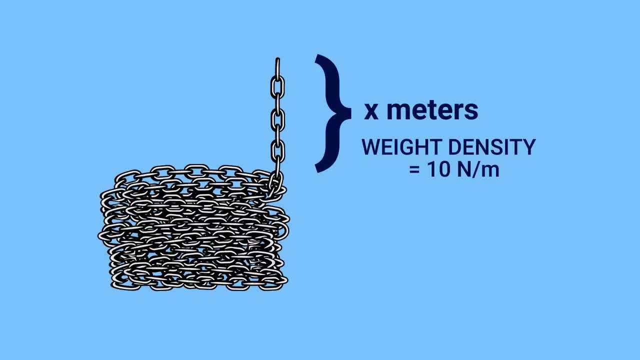 density of 10 N per meter. Thus the weight of just the section off the ground is 10x. So if the chain were 2 meters off the ground then you'd have to use a force of 20 N to hold it in place. 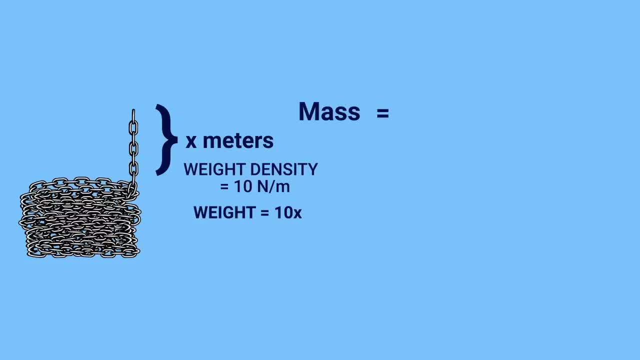 Then the equation for mass for the part of the chain off the ground is simply the weight divided by gravity. Weight is 10x, and I'll round gravity to 10, as always. So the mass of this part of the chain off the ground is just x. 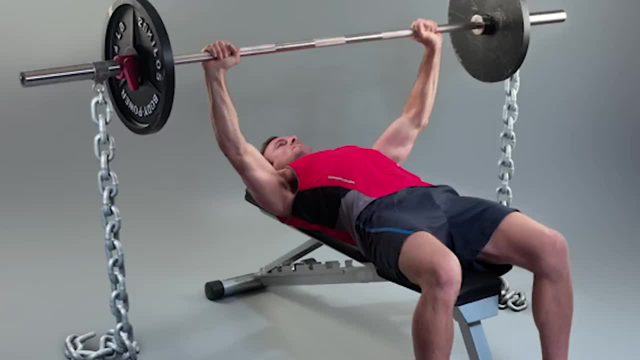 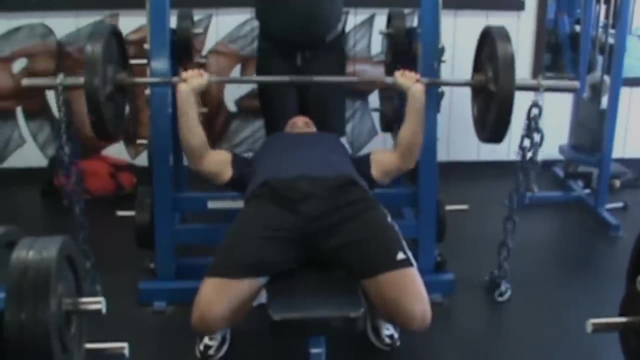 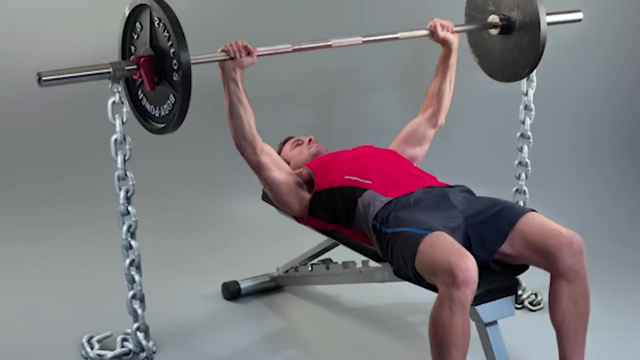 This makes it so that, as the bar moves up, the chain is more and more suspended and thus contributes more of its weight to the exercise Meaning. as the person pushes upwards, the weight increases. This actually complicates the equation of motion more than you might think, because 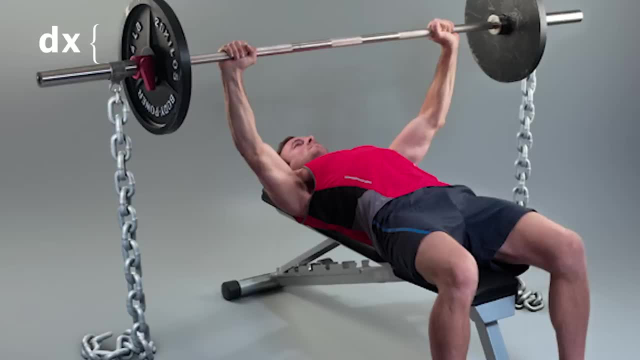 for every little dx or change in height, there's a dm or small change in mass in regards to the part of the chain that's off the ground. So let's see what this setup would look like. Now we'll say the barbell has no mass. 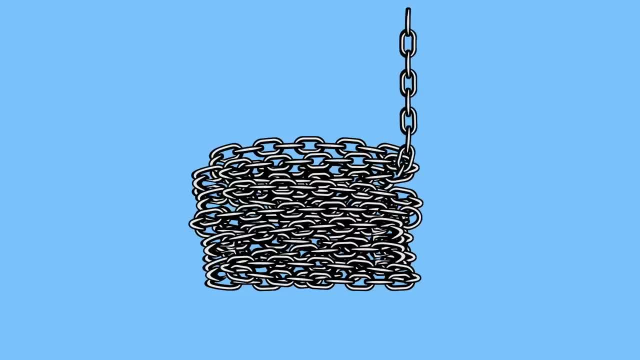 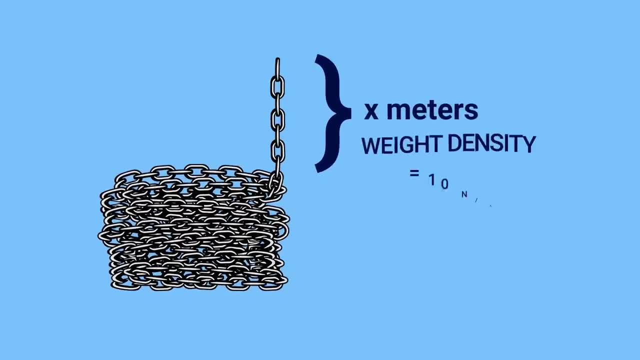 just to make things easier. so really we're just lifting the chain off the ground and we'll call that distance off the ground x, measured in meters. Then let's give the chain a weight density of 10 N per meter, Thus the weight of just the section off the ground. 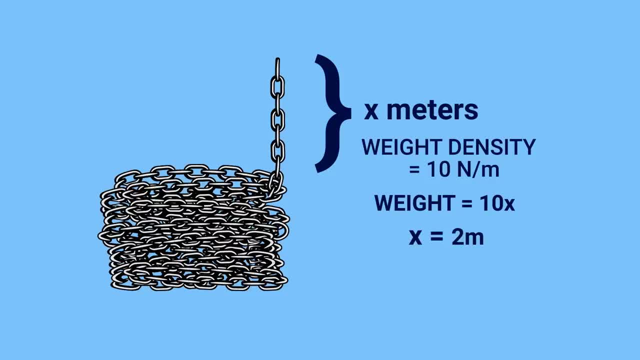 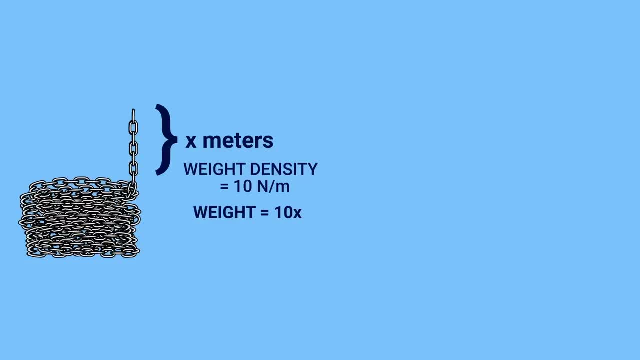 is 10x. So if the chain were 2 meters off the ground then you'd have to use a force of 20 N to hold it in place. Then the equation for mass for the part of the chain off the ground is simply the weight. 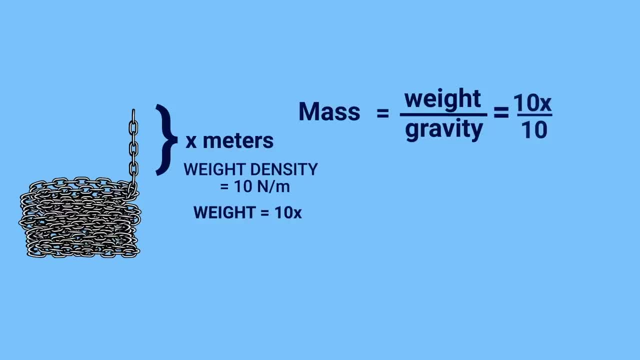 divided by gravity, Weight is 10x, and I'll round gravity to 10, as always. so the mass of this part of the chain off the ground is just x. Lastly, we'll say the person is pushing up with a constant force. 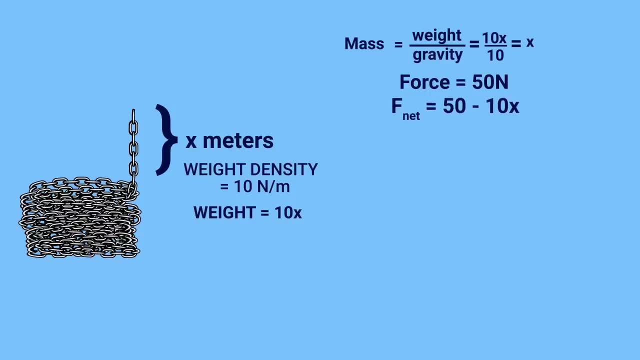 of 50 N, meaning the net force is 50 up minus the 10x down from the chain itself. Okay now, before we can move on, we have to realize that F equals ma is a lie. Well, not really, But it only applies to special cases. 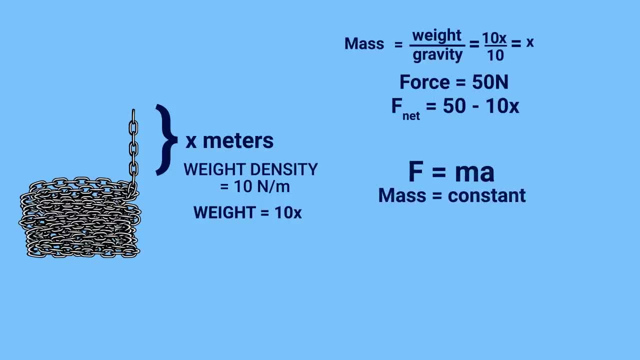 where the mass is constant. The real equation we have to work with is: F equals the rate of change of momentum or mass times, velocity, Doing a simple product rule. we get this here And you'll notice when m is not changing, which. 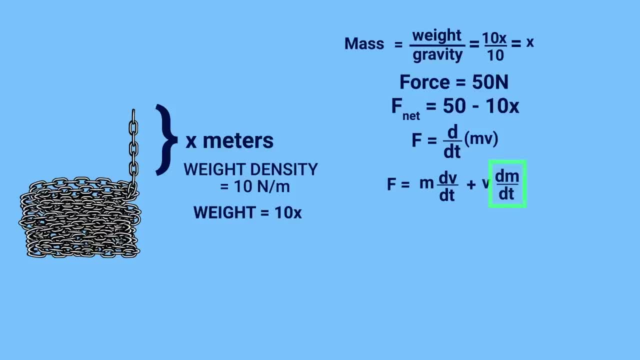 we get used to in a first level physics course. then this term is zero And we're left with F equals m, times dv, dt or F equals ma, as usual, But with the changing mass we have this entire equation From here. I'm just going to replace the 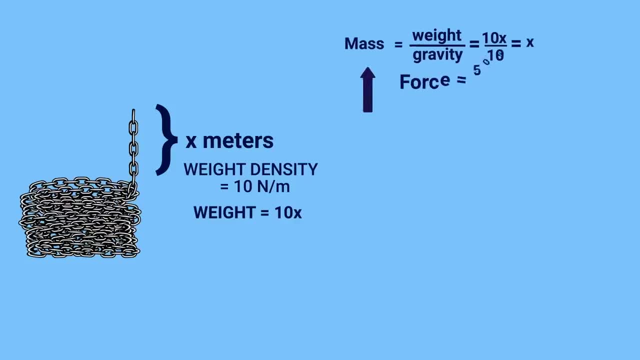 Lastly, we'll say: the person is pushing up with a constant force of 50 N, Meaning the net force is 50 up minus the 10x down from the chain itself. Okay, now, before we can move on, we have to realize that F equals ma is a lie. 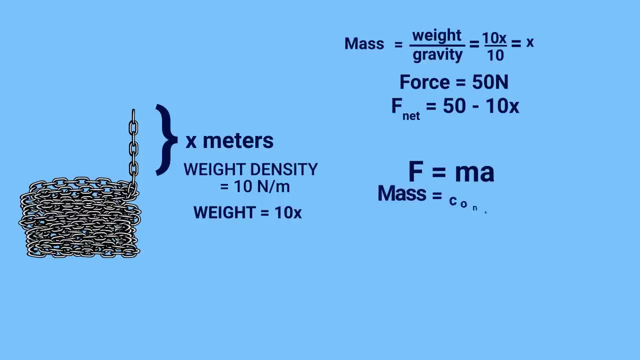 Well, not really, But it only applies to special cases where the mass is constant. The real equation we have to work with is: F equals the rate of change of momentum or mass times velocity, Doing a simple product rule. we get this here And you'll notice when m 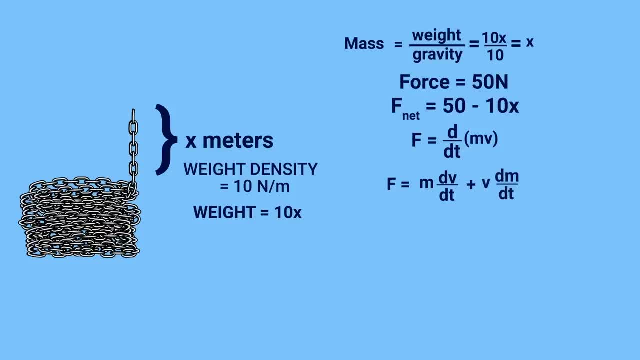 is not changing, which we get used to in a first level physics course. then this term is 0 and we're left with F equals m times dv, dt or F equals ma, as usual, But with the changing mass we have this entire equation. 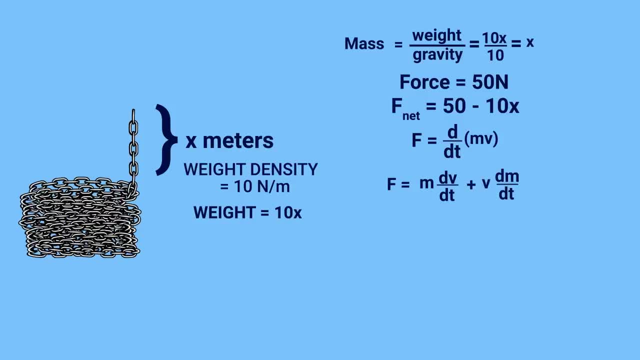 From here. I'm just going to replace the variables like: mass is really x and force is 50 minus 10x. So we get this here. But velocity is just the rate of change of position and dv, dt, which is acceleration, is the second derivative of position. 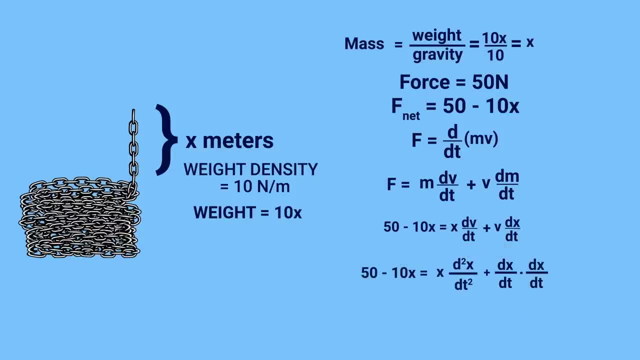 So we're left with this equation here Moving the 10x over. we're left with a second order, non-linear differential equation. Solving this would not be easy, but not really the point of this video. Instead, I just want to highlight that the motion which results: 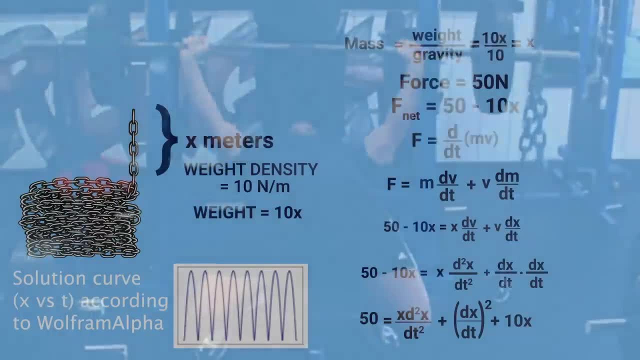 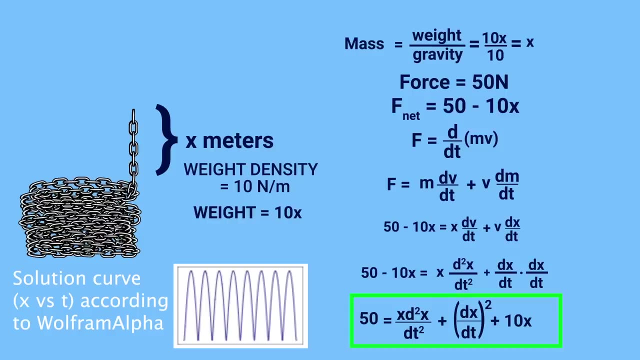 by something as simple as pulling a chain upwards, has to be expressed through a not so simple second order differential equation, And while it may be true that analyzing the motion of a barbell isn't too applicable, the idea of analyzing a system with changing mass, 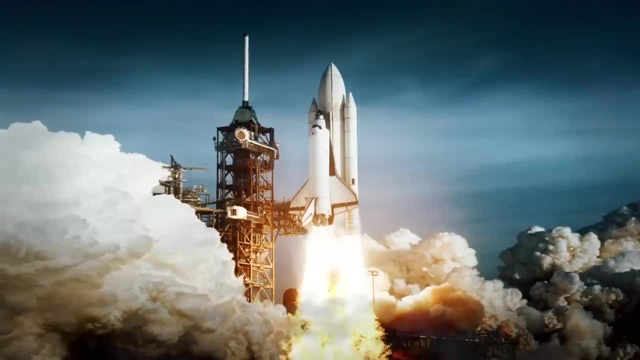 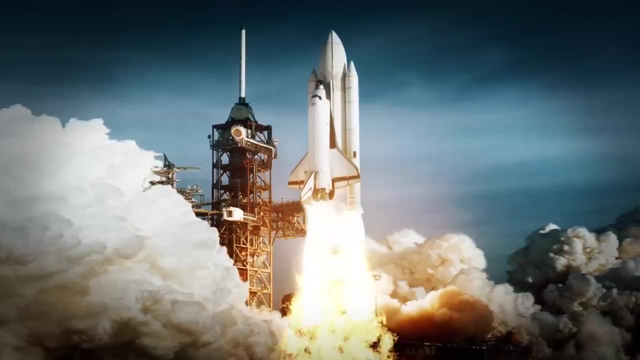 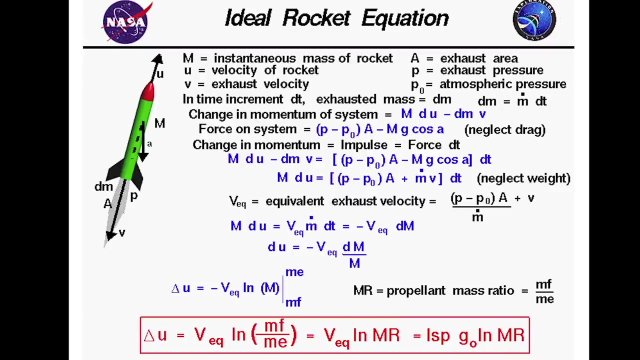 is The perfect example is a rocket. As exhaust leaves the bottom, the rocket itself loses mass little by little. So thrust and a changing mass are kind of linked And the situation also leads to differential equations. But now let's look at the most real world application. 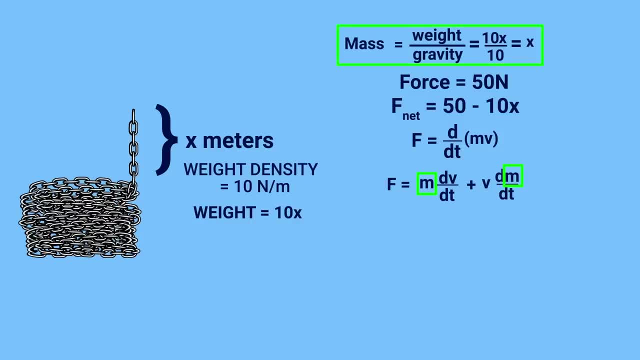 variables like mass is really x and force is 50 minus 10x, So we get this here. But velocity is just the rate of change of position and dv dt, which is acceleration, is the second derivative of position. So we're left with 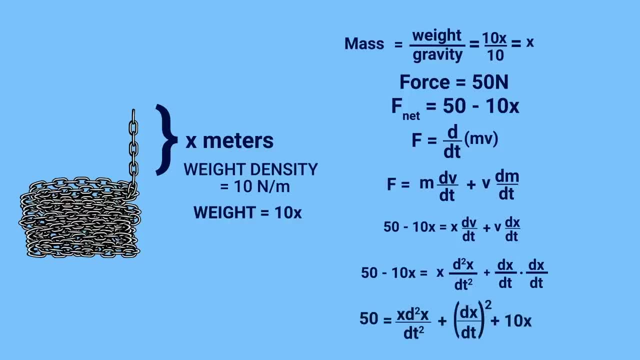 this equation here. Moving the 10x over, we're left with a second order non-linear differential equation. Solving this would not be easy, but not really the point of this video. Instead, I just want to highlight that the motion which results by something as simple 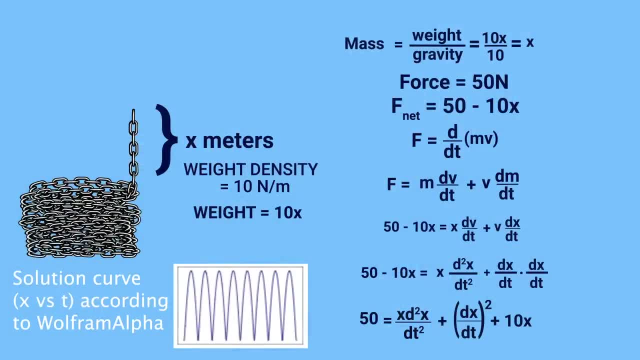 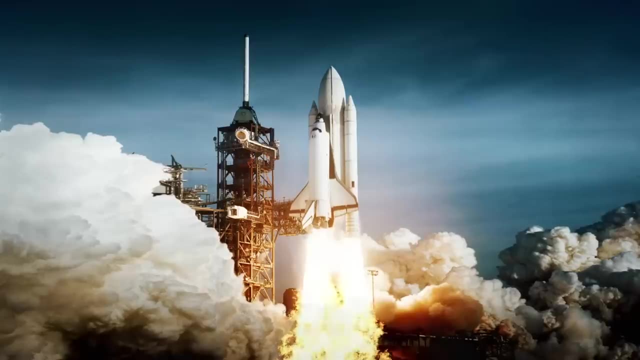 as pulling a chain upwards, has to be expressed through a not so simple second order differential equation, And while it may be true that analyzing the motion of a barbell isn't too applicable, the idea of analyzing a system with changing mass is The perfect example is a rocket. 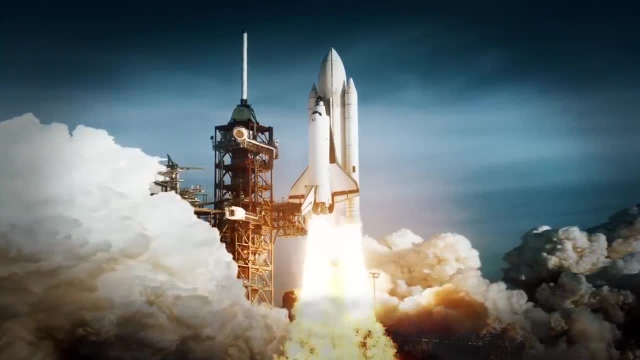 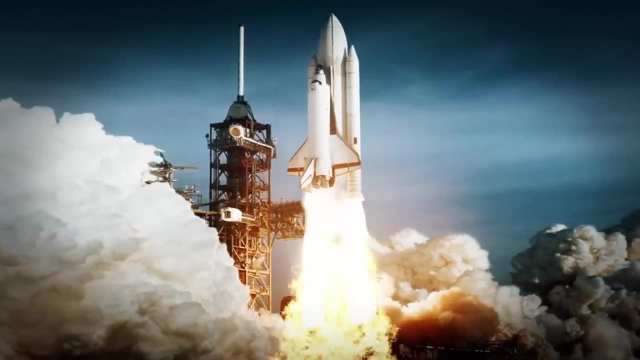 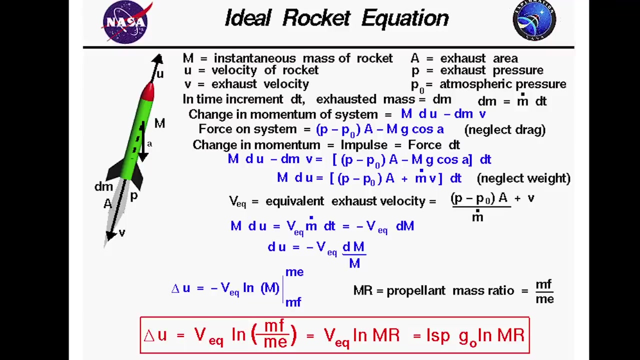 As exhaust leaves the bottom, the rocket itself loses mass little by little. So thrust and a changing mass are kind of linked, and the situation also leads to differential equations. But now let's look at the most real world application I can think of. 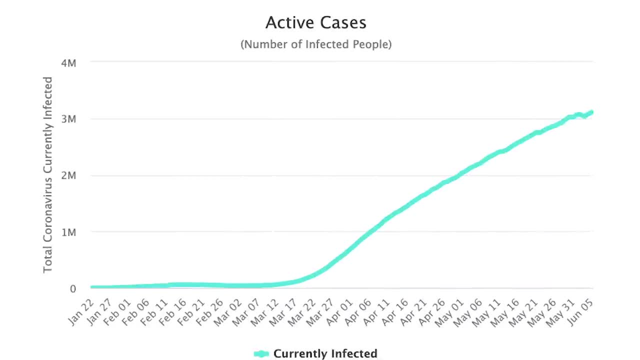 This here is a curve of the number of currently infected people from the coronavirus as of early June. It's infected people versus time, which means the instantaneous rate of change or slope at any point is di dt. It gradually increased for a while before flattening out, but we want that. 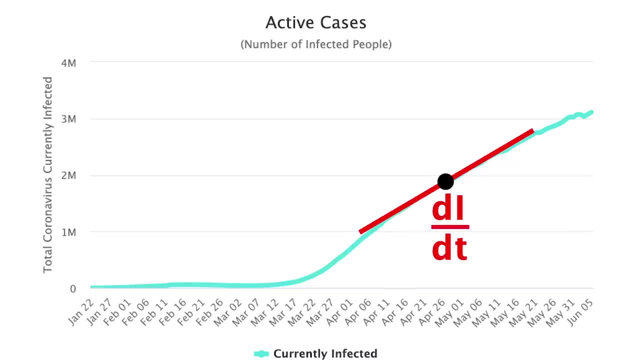 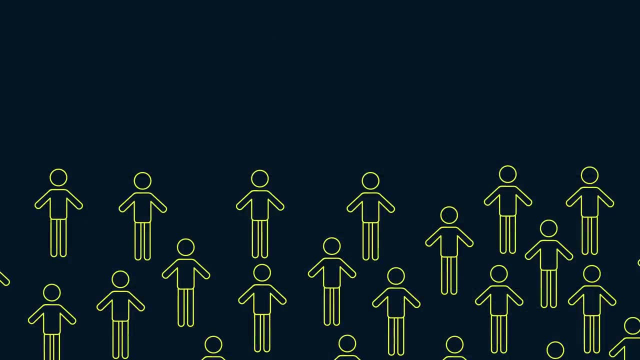 rate of change to go negative. Anyways, this is an incomplete picture of what's going on, because there are other categories of people out there In the population. there are those that have never been infected or those that are susceptible, Those that are currently infected. 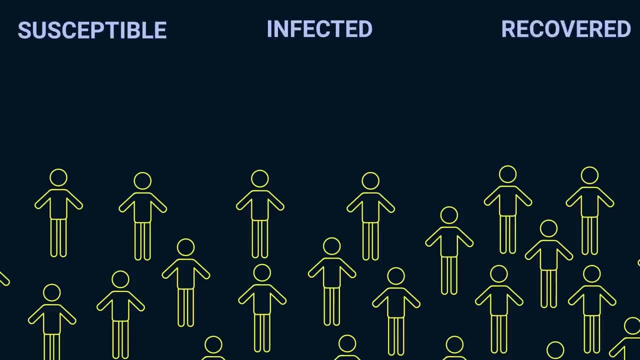 and then those that are recovered or, unfortunately, deceased. But the most basic model, the SIR model, just calls it recovered and assumes no deaths. I know many YouTubers have talked about this recently so I'll keep it kind of short. 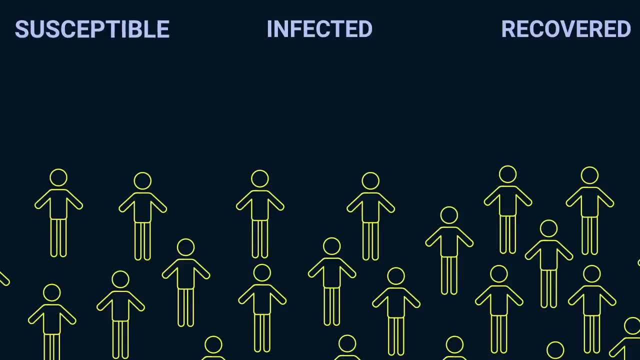 In the case of the coronavirus, everyone started in the susceptible bucket And let's say the population is 20. So no one is infected, but everyone has the potential to be, And then one day one person transitioned to infected. This was basically an initial condition. 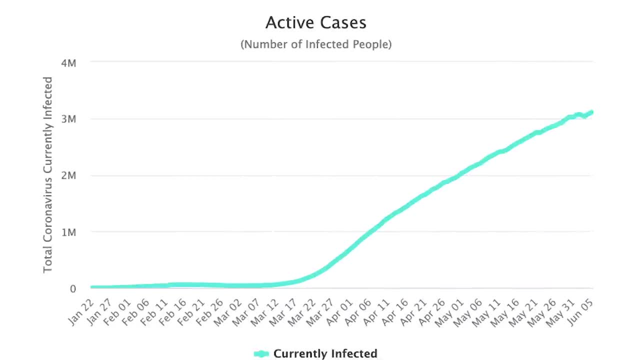 I can think of This. here is a curve of the number of currently infected people from the coronavirus as of early June. It's infected people versus time, which means the instantaneous rate of change or slope at any point is: did It gradually increased for a while before flattening out? 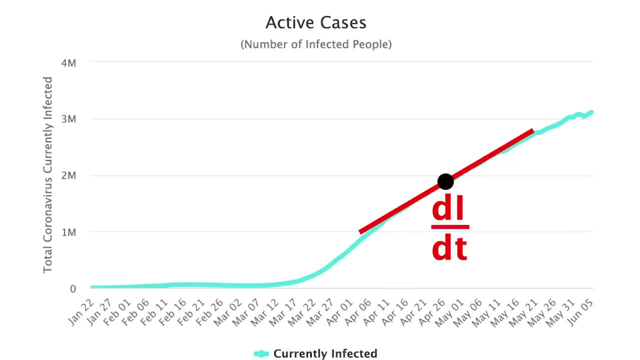 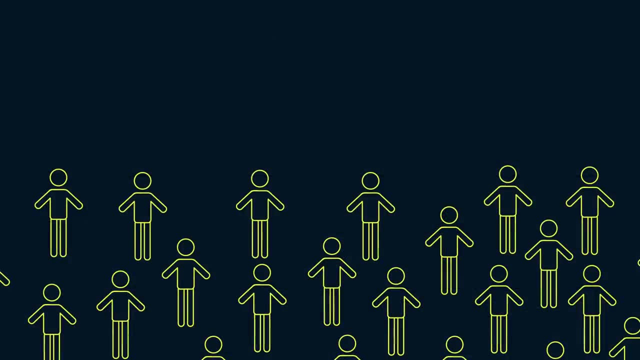 but we want that rate of change to go negative. Anyways, this is an incomplete picture of what's going on, because there are other categories of people out there In the population. there are those that have never been infected or those that are susceptible, those that 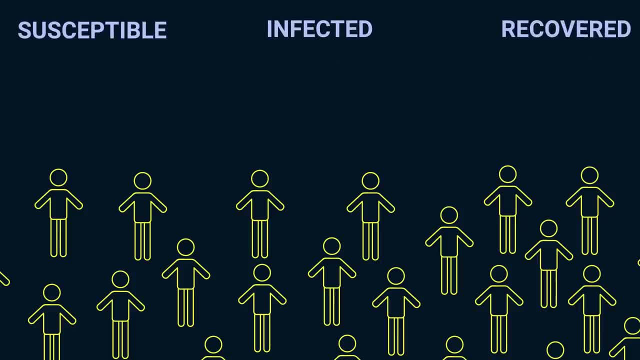 are currently infected, and then those that are recovered or, unfortunately, deceased. But the most basic model, the SIR model, just calls it recovered and assumed no deaths. I know many YouTubers have talked about this recently so I'll keep it kind of short. In the case, 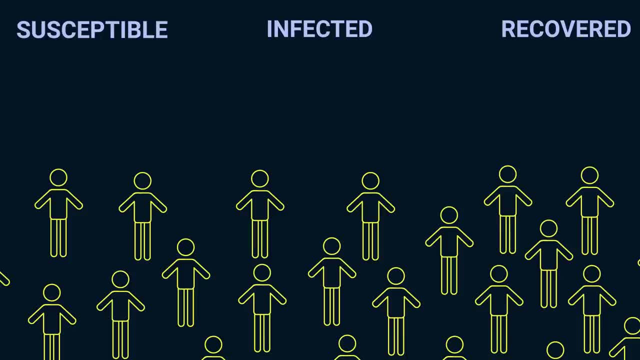 of the coronavirus. everyone started in the susceptible bucket And let's say the population is 20. So no one is infected, but everyone has the potential to be, And then one day one person transitioned to infected. This was basically an initial condition. 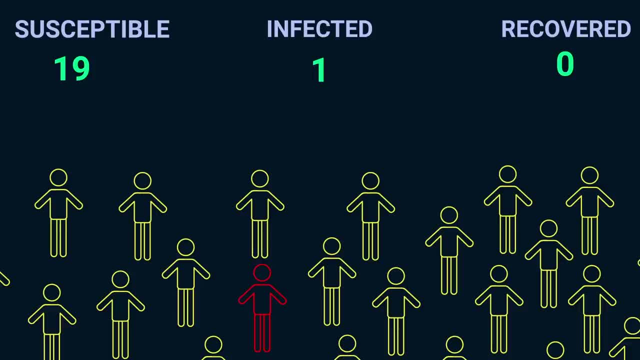 Now, if the population stays constant, no one new is born, then the number of susceptible people can only go down or stay the same, Because as soon as you get infected you leave that group never to return, Assuming immunity after you get the disease. 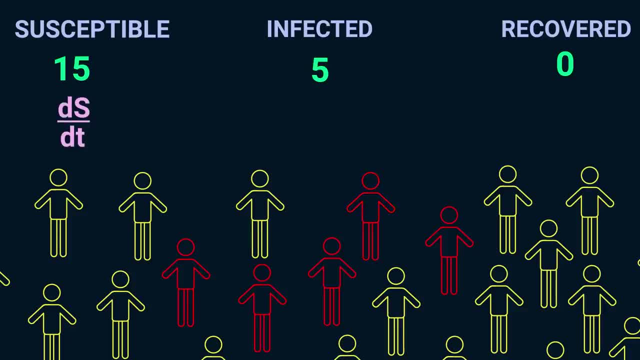 So the rate of change of susceptible people is going to be negative, something It can only go down, Since having a lot of infected people or a lot of susceptible people slash a high population, increases the magnitude of that change. then we say it's S times I. 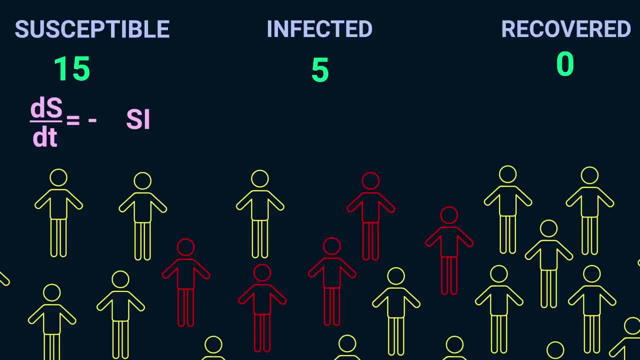 Where S and I are the number of susceptible and infected people respectively. If either of these are large and the other is non-zero, you have a large transition to those who are infected. But we also have to include a constant. That constant depends on. 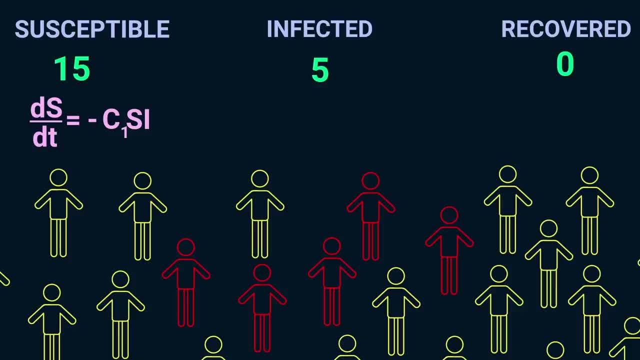 the virus and us As it scales how quickly people go from healthy to sick. Social distancing or hand washing, for example, would decrease that constant and this rate of change wouldn't be as extreme. Then the rate of change of those who are infected starts with that same expression seen. 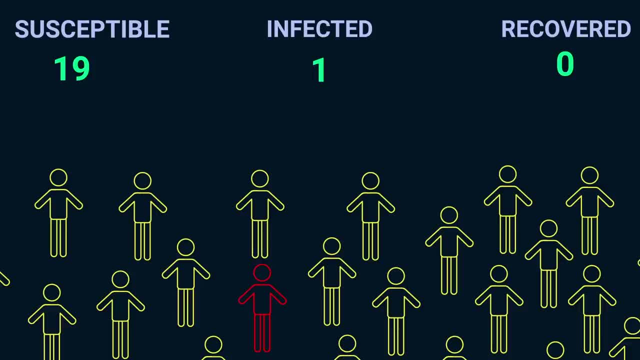 Now, if the population stays constant, no one new is born, then the number of susceptible people can only go down or stay the same, Because as soon as you get infected you leave that group never to return, Assuming immunity after you get the disease. 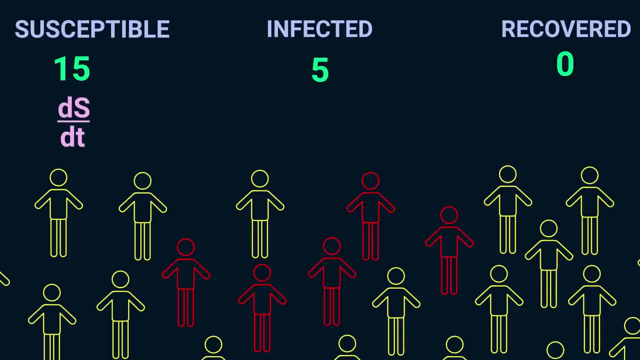 So the rate of change of susceptible people is going to be negative, something It can only go down, Since having a lot of infected people or a lot of susceptible people in a high population increases the magnitude of that change. then we say it's S times I. 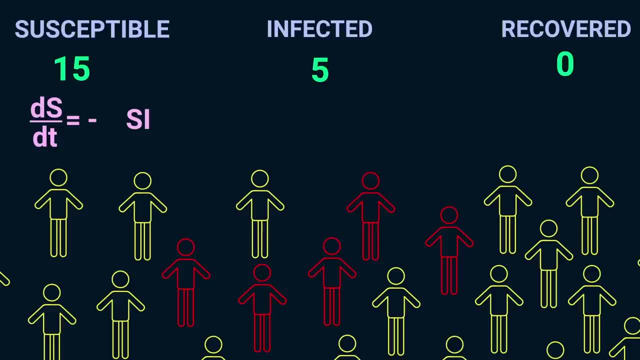 Where S and I are the number of susceptible and infected people respectively. If either of these are large and the other is non-zero, you have a large transition to those who are infected. But we also have to include a constant. That constant depends on the virus and 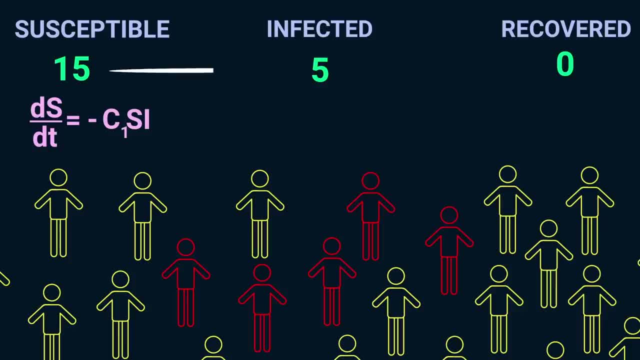 us as it scales how quickly people go from healthy to sick. Social distancing or hand washing, for example, would decrease that constant and this rate of change wouldn't be as extreme. Then the rate of change of those who are infected starts with that same expression. 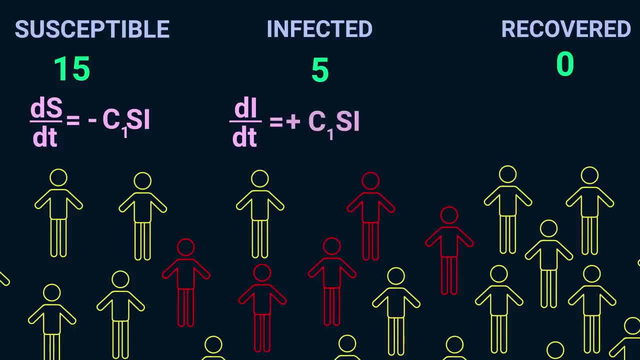 seen on the left, but positive. This is because in this model it's a one-way street. If someone leaves the susceptible pile, they go to infected, But people will leave the infected pile proportional to how many infected people there are. 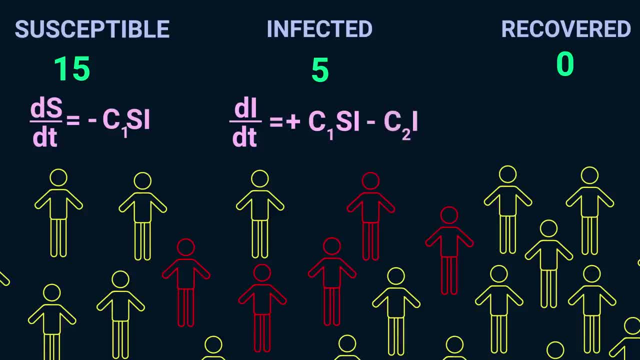 This constant in reality is death rate combined with recovery rate. If medicine is released that speeds up recovery by 50%, then that constant goes up and people are quicker to leave the infected pile and become recovered. The rate of change of those who have 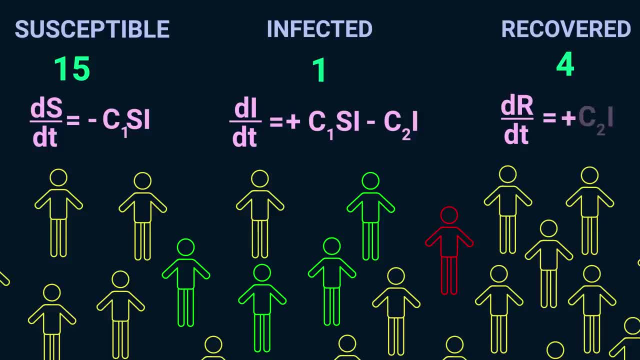 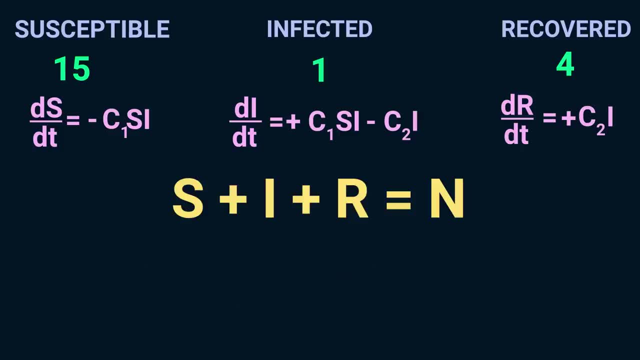 recovered can only be positive or zero, and it's that same constant times. I You'll notice in this model that we kept the population constant, so the sum of the three categories was always the same, meaning the rates of change should add to zero, as they do. 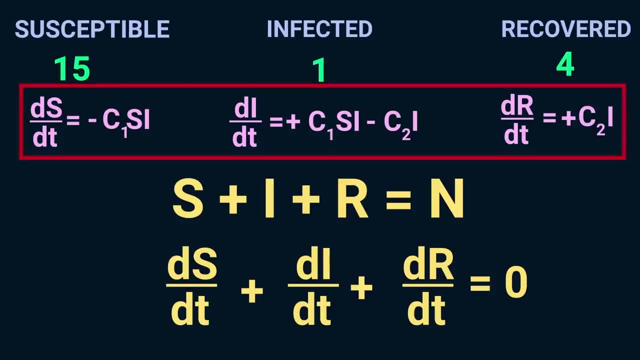 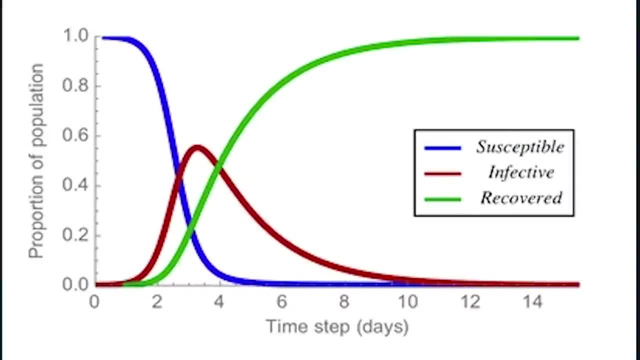 But here we're left with another system of differential equations that, when solved, will tell you how an infection will spread through a population in this simplified scenario. I'm sure many of you have seen Numberphile's video on this that I'll link below. but there you. 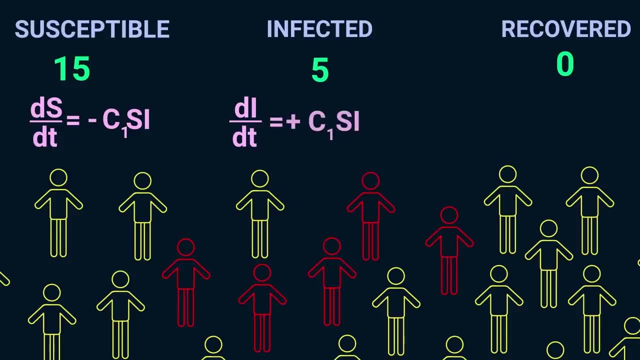 on the left, but positive. This is because in this model it's a one way street. If someone leaves the susceptible pile, they go to infected, But people will leave the infected pile proportional to how many infected people there are. This constant in reality is: 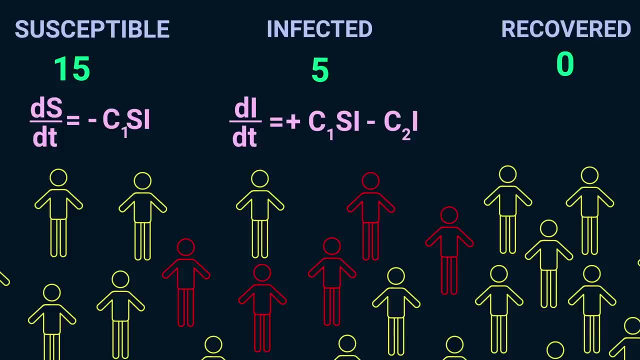 death rate combined with recovery rate. If medicine is released that speeds up recovery by 50%, then that constant goes up and people are quicker to leave the infected pile and become recovered. The rate of change of those who have recovered can only be positive or zero. 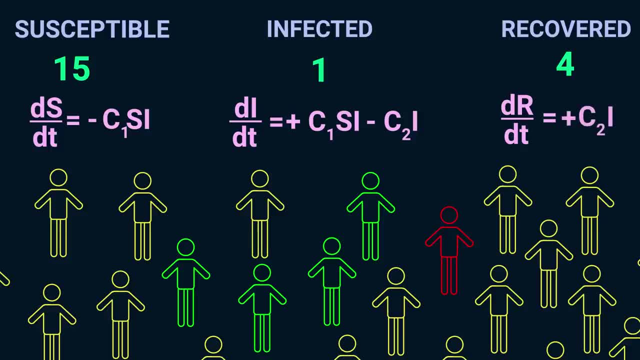 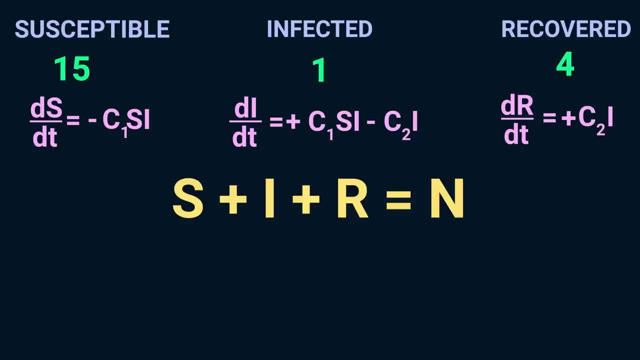 and it's that same constant times. i You'll notice in this model that we kept the population constant, so the sum of the three categories was always the same, meaning the rates of change should add to zero, as they do. But here we're left with another system. 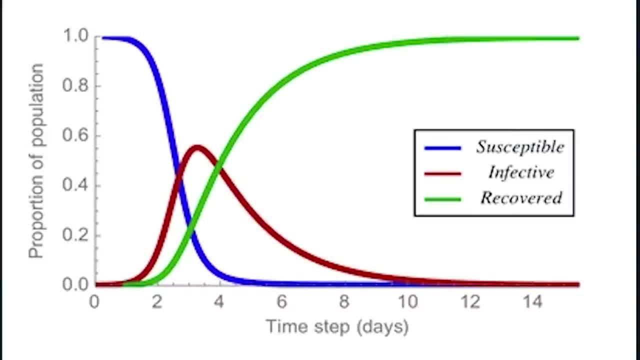 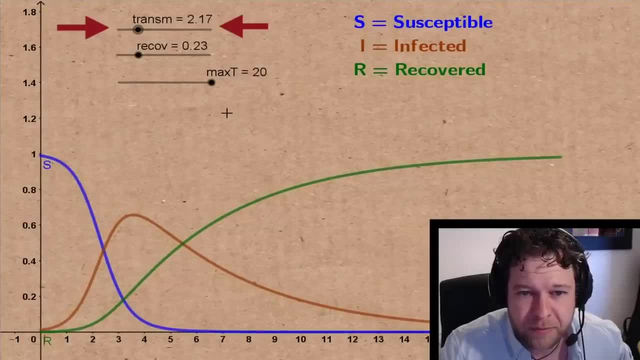 of differential equations that, when solved, will tell you how an infection will spread to the population in this simplified scenario. I'm sure many of you have seen Numberphile's video on this that I'll link below, but there you can see what happens when you play around with the equations. 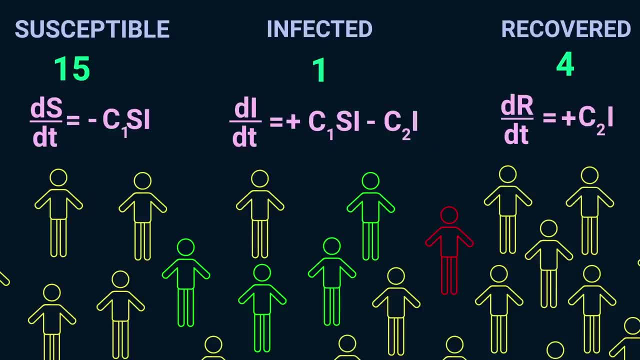 and constants and all that. As with most of these examples, we did simplify things to make the math easier, but this is all the foundations of what's going on in the real world. If you go to the website for the International Council for Industrial and Applied Mathematics, 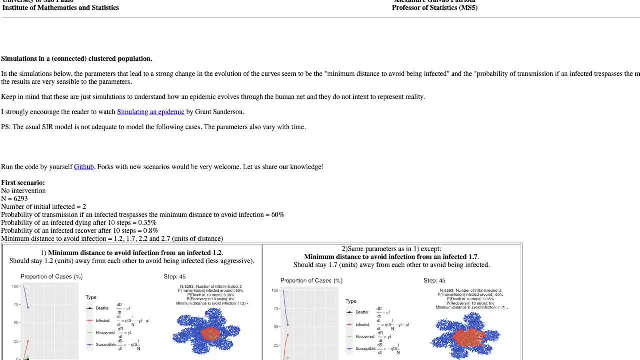 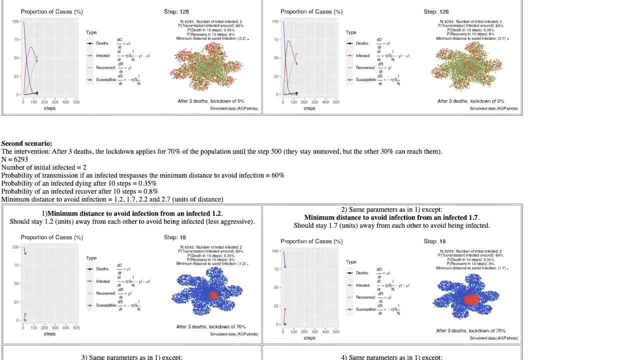 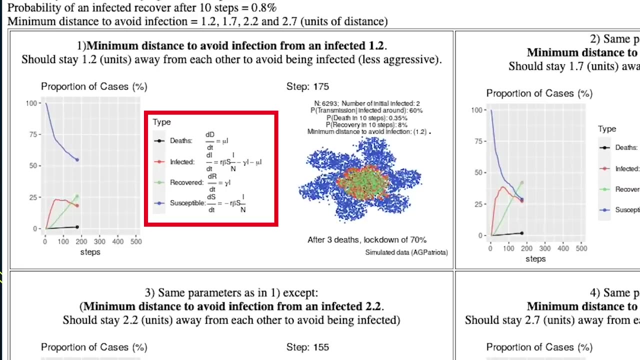 there's a page on the mathematics of COVID-19 showing the simulations and models that mathematicians are creating to understand the spread of this virus in different parts of the world, where you'll find equations just like we saw. Equations very similar to these also show up in terms of. 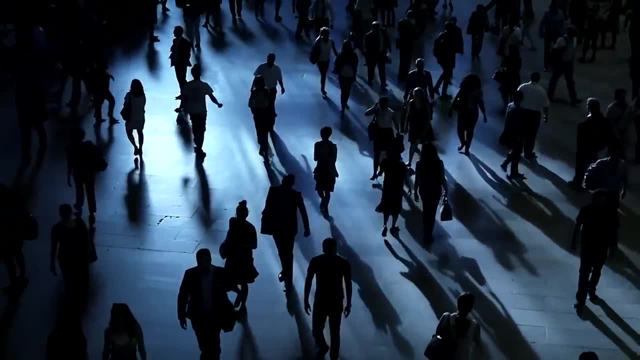 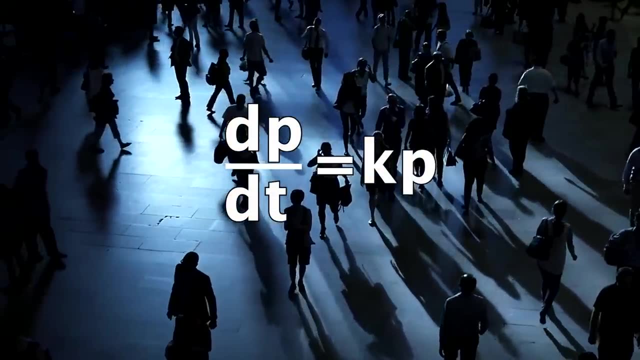 population growth. One of the first differential equations a lot of us learn is the one that models how a population will grow at a rate proportional to its current value. The more people or animals there are, the faster the growth, as expected. Things get more complicated with deaths. 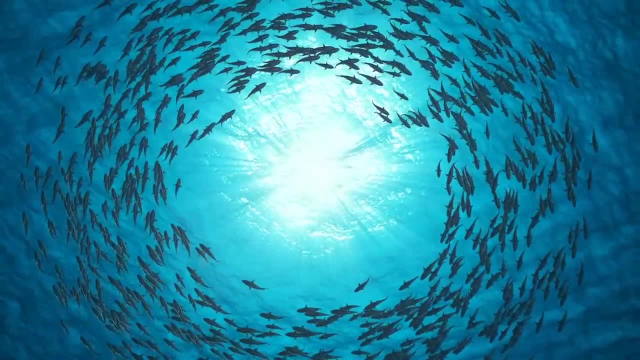 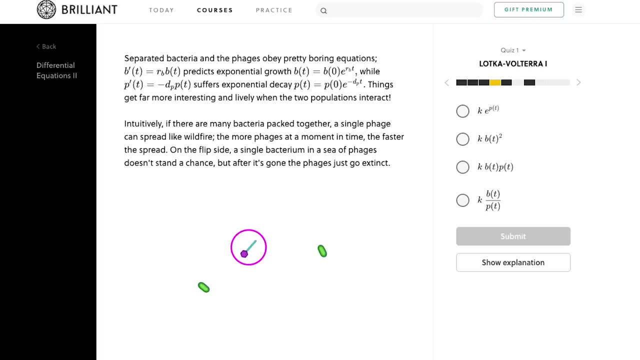 or when maybe one population kills off another. Here's an example of bacteria which can multiply on their own and phages that essentially feed off bacteria and thus will die without them, And you'll see that after one cycle here the phages grow from one to four. 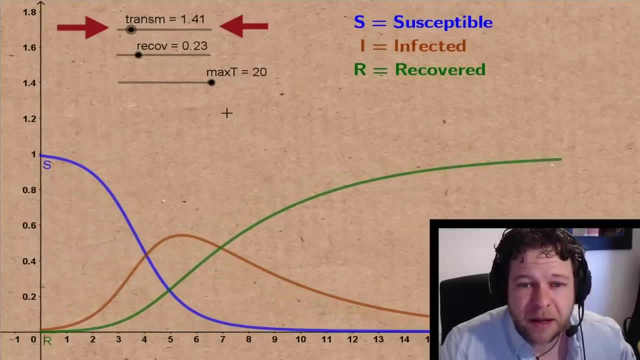 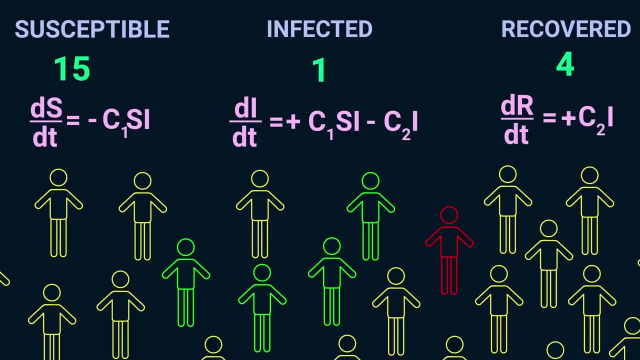 can see what happens when you play around with the equations and constants and all that. As with most of these examples, we did simplify things to make the math easier, but this is all the foundations of what's going on in the real world. If you go to the website, 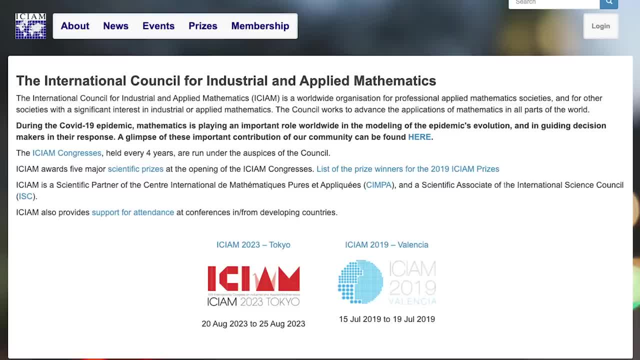 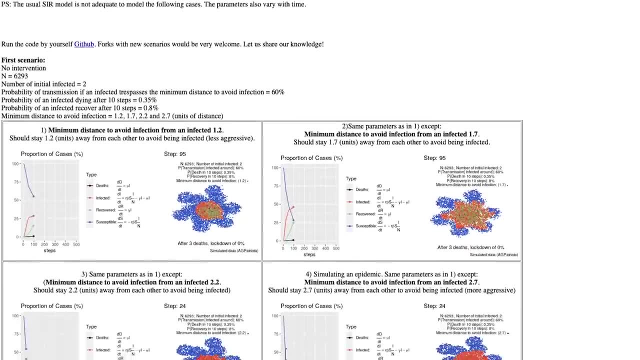 for the International Council for Industrial and Applied Mathematics, there's a page on the mathematics of COVID-19, showing the simulations and models that mathematicians are creating to understand the spread of this virus in different parts of the world, where you'll find equations just 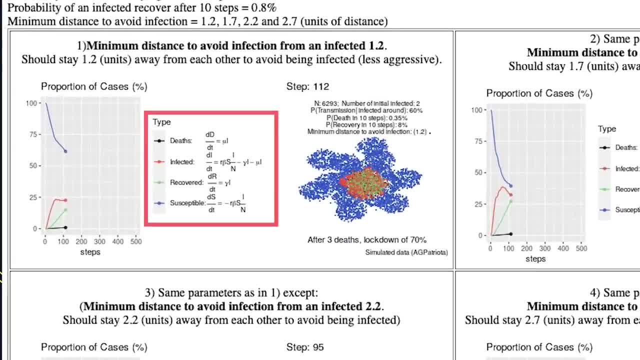 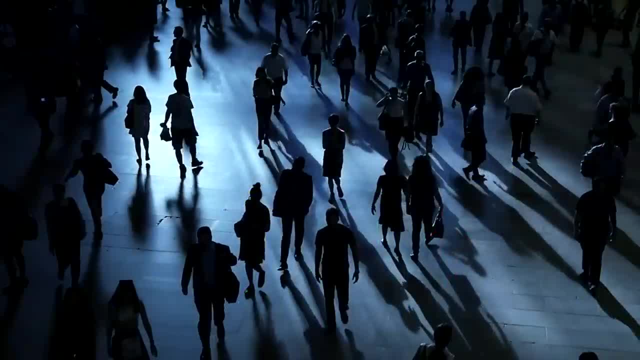 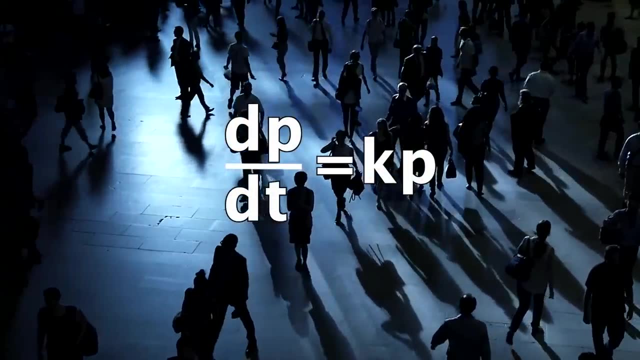 like we saw. Equations very similar to these also show up in terms of population growth. One of the first differential equations a lot of us learn is the one that models how a population will grow at a rate proportional to its current value, The more people or animals there are. 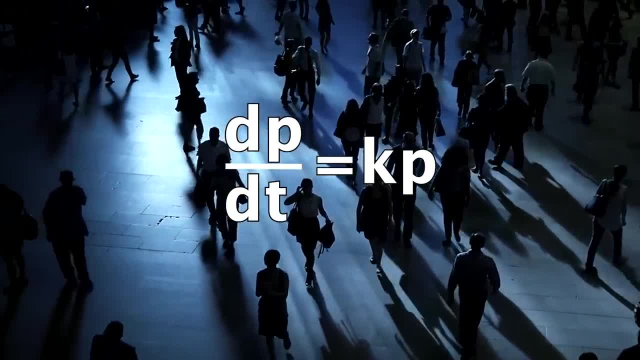 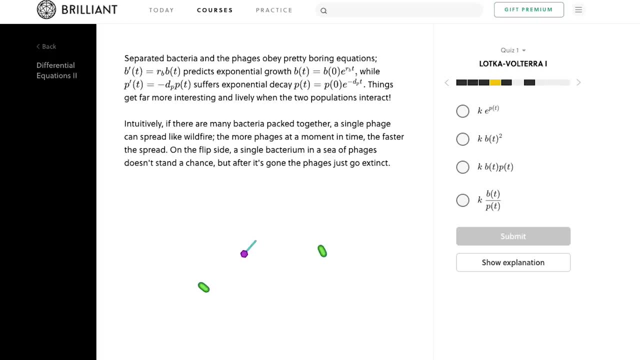 the faster the growth, as expected, But things get more complicated with deaths or when maybe one population kills off another. Here's an example of bacteria which can multiply on their own and phages that essentially feed off bacteria and thus will die without them. 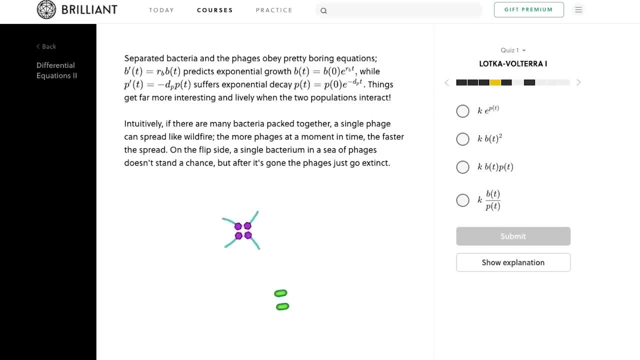 And you'll see that after one cycle here the phages grow from one to four, but the bacteria stay at two, And now there are more phages. so some will die while others will continue to multiply. So there's kind of this back. 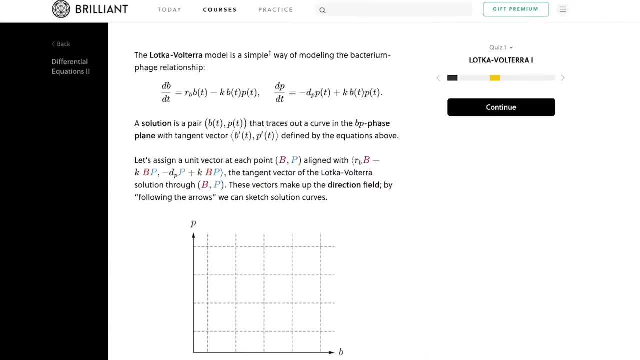 and forth. that happens, but it leads to differential equations where the rates of change depend on multiples of the populations. And it's not always about just solving the equations, as there are tools such as phase portraits that can help paint a picture about what's going. 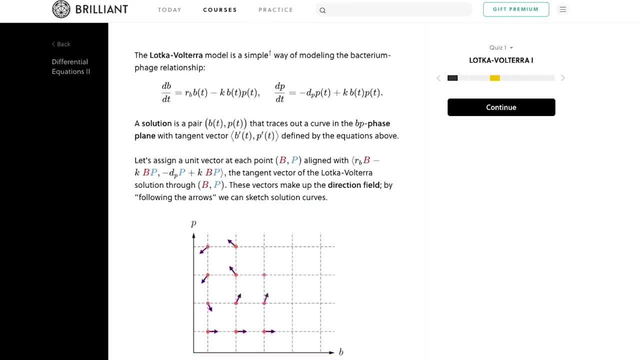 on without having to find an actual solution Here. if you're given a certain population of phages and bacteria, this would tell you how the system, or really both populations- will change at that moment, And with this we can find equilibrium points or long term. 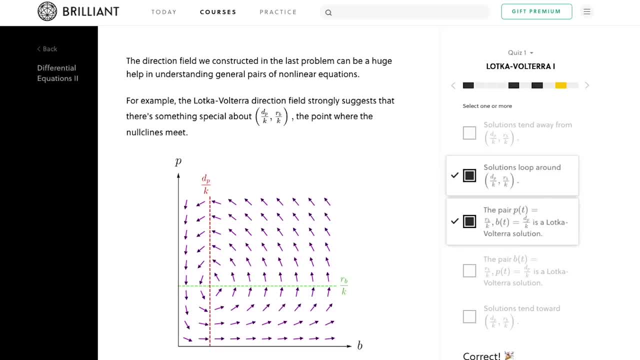 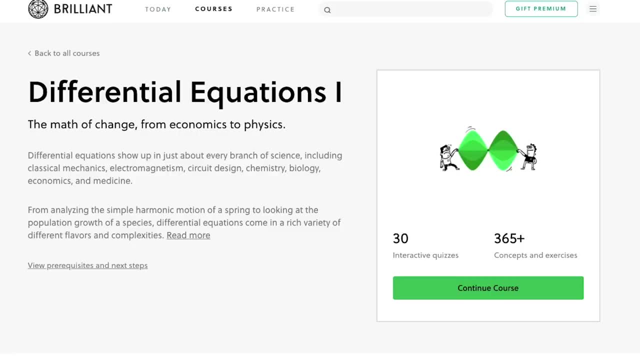 behavior, for example, And while I'm not going to go any further than this, I think we've discussed a lot. if you want to dive more into the topic of differential equations, you can, of course, do so right here at Brilliant. Currently, they have two differential equations. 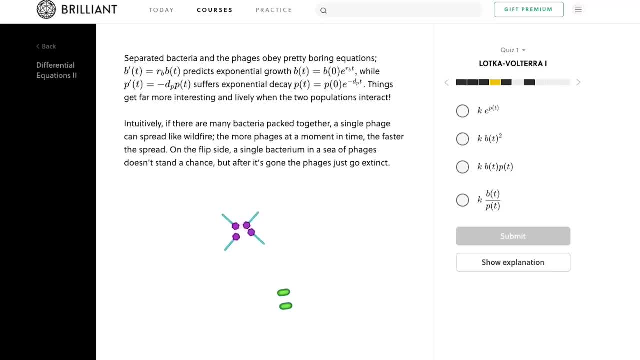 but the bacteria stay at two, And now there are more phages, so some will die while others will continue to multiply. So there's kind of this back and forth that happens, but it leads to differential equations where the rates of change depend on multiples of the populations. 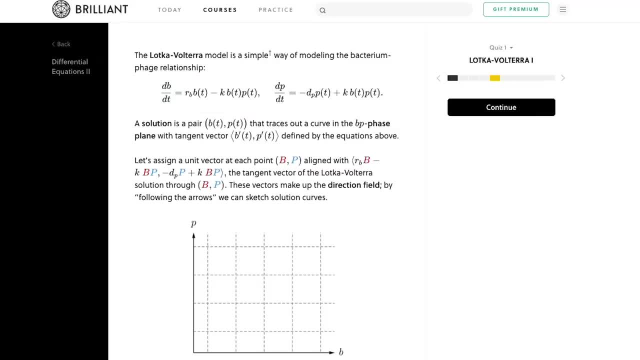 And it's not always about just solving the equations, as there are tools such as phase portraits that can help paint a picture about what's going on without having to find an actual solution Here. if you're given a certain population of phages and bacteria, this would tell you how. 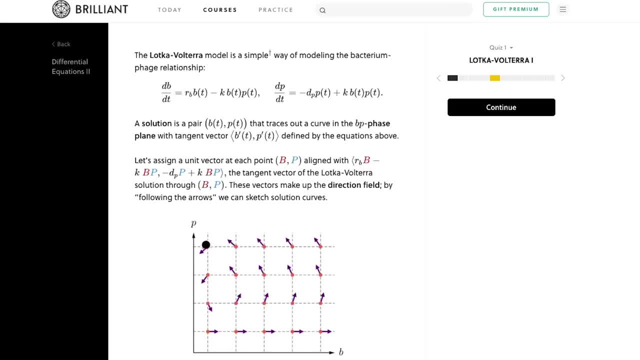 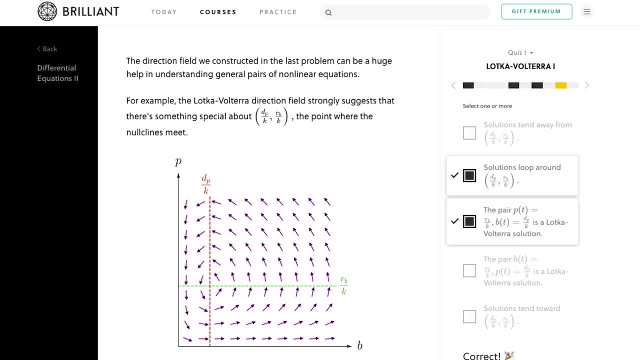 the system, or really both populations, will change at that moment And with this we can find equilibrium points or long term behavior, for example, And while I'm not going to go any further than this, I think we've discussed a lot if you want to dive more into the topic. 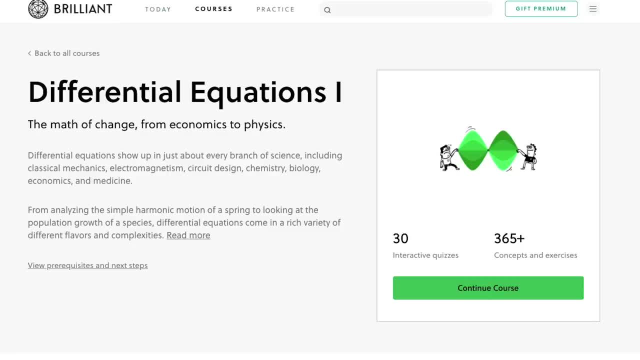 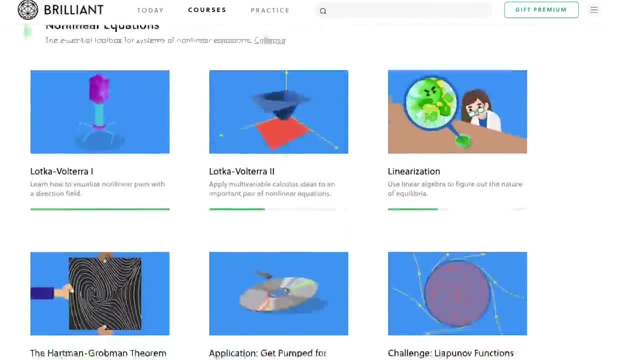 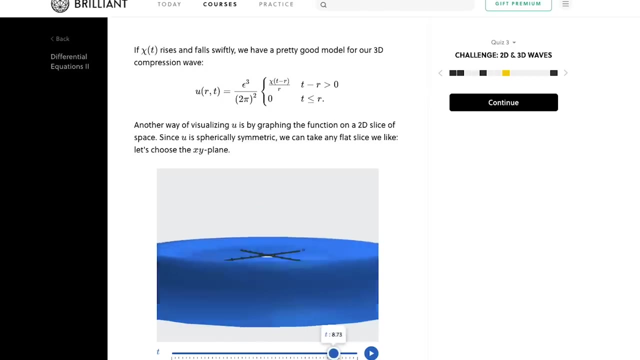 of differential equations. you can, of course, do so right here at Brilliant. Currently they have two differential equations courses, which are some of my favorites because of how much they focus on real world applications. They have the pursuit curves we discussed. there's 2D and 3D wave equations. 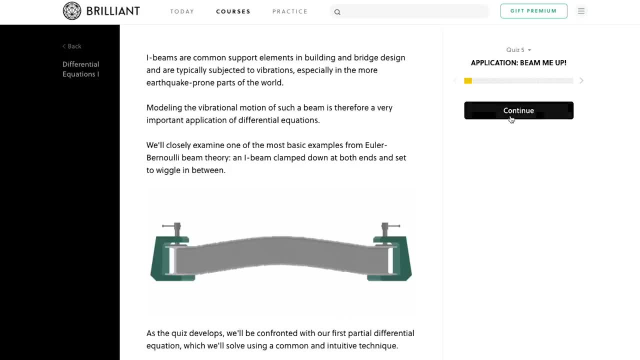 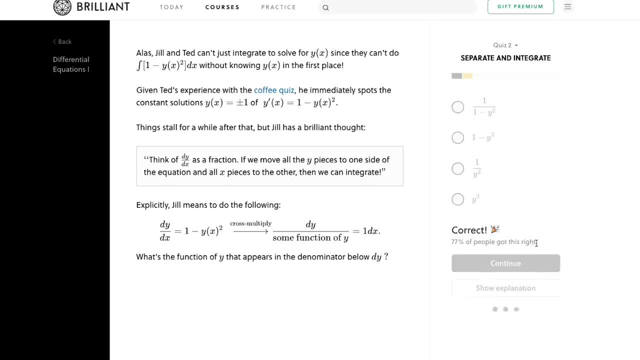 there's the equations that model the behavior of beams and much more. Their first course does start at the basics for anyone just starting out, but by the second course there are things I never saw as an engineer in college. so regardless of where you are in your education, 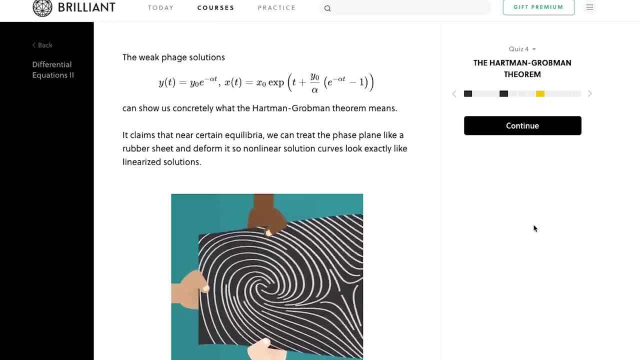 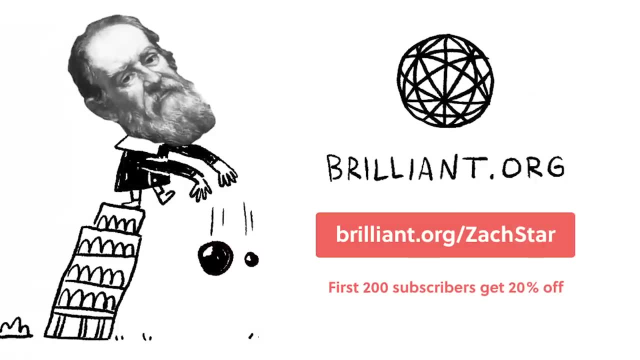 there likely is a lot to learn, whether you want to get ahead as a student or just brush up on old topics. So if you want to get started right now and support the channel, you can click the link below or go to brilliantorgsacstar. 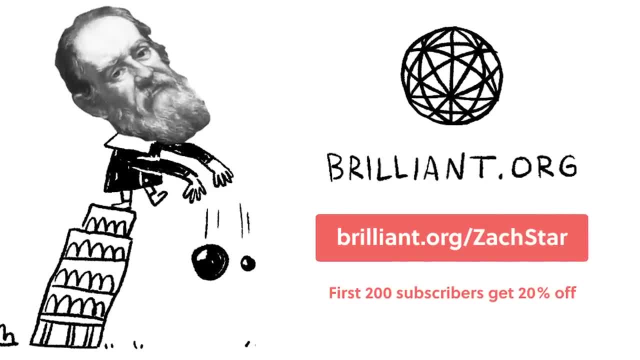 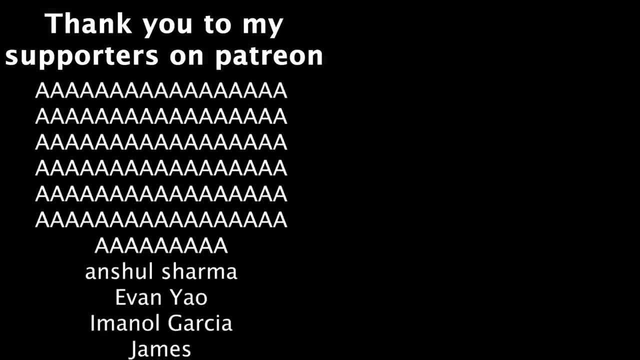 plus, the first 200 people to sign up will get 20% off their annual premium subscription. And with that I'm going to end that video there. Thanks, as always, to my supporters on Patreon. social media links to follow me are down below and I'll see you guys in the next video.